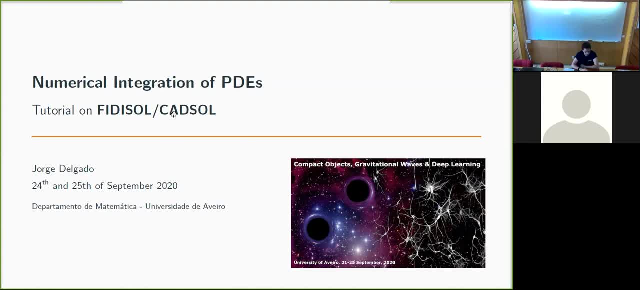 I will just call CatSolve, just to be a bit more easier. So in this first lecture I will speak and try to explain a bit how CatSolve solver works, and we will also obtain a numerical care solution. In the next lecture tomorrow I'll give you a boson star, a scalar boson star with rotation solution. 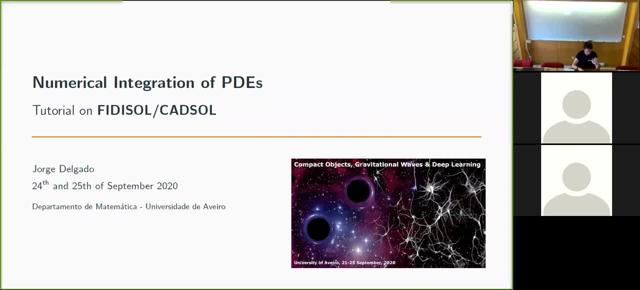 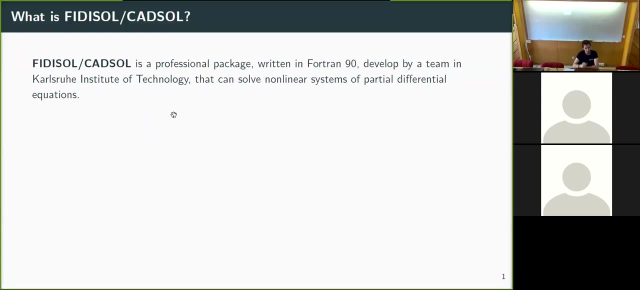 and with that solution, we'll use it to obtain physical quantities such as mass, angular momentum and other quantities. So let's begin. So what is CatSolve? What is this solver? It's a professional package written in 1419, that was developed by a team in Karlsruhe, if I'm not mistaken by the name. 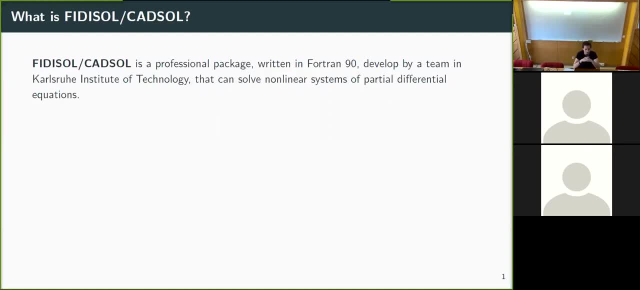 and can solve non-linear systems of partial differential equations. These differential equations can be two- or three-dimensional, they can be elliptic or parabolic and they can be subject to arbitrary boundary conditions. on a rectangular domain, The solver uses a finite difference method, which is a Newton-Raphson method. 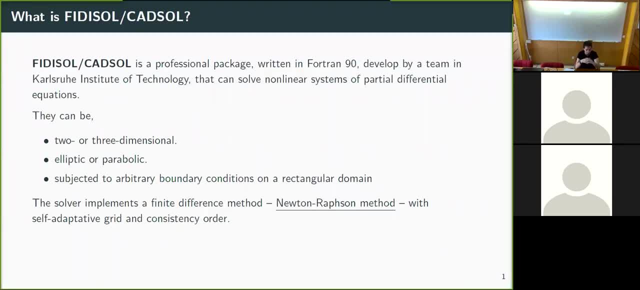 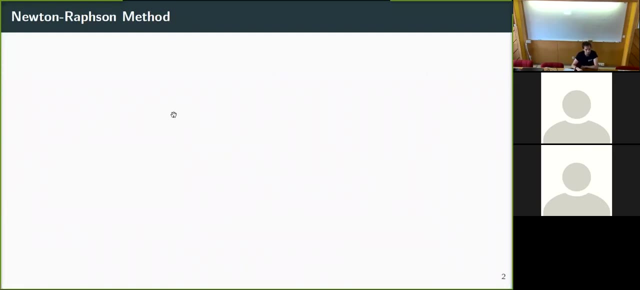 and can use self-adapting grid and some arbitrary conditions. The solver also provides- it's quite a feature of the solver- error estimations for the compute solution. So just to remind what is the Newton-Raphson method for those who don't remember: 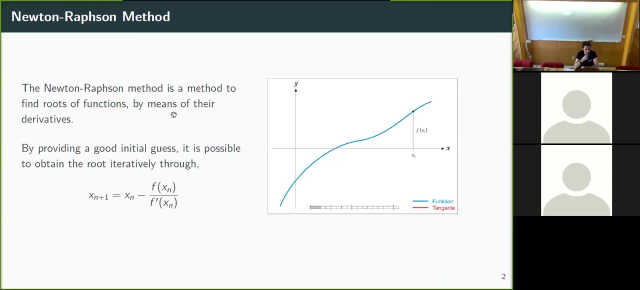 it's a very simple method to find the roots of some function by using the derivative of that function. You can obtain the root by implementing this equation iteratively, as you can see by the animation. But this method also can find functions, And this is what Fitts-Solve or Katz-Solve does. 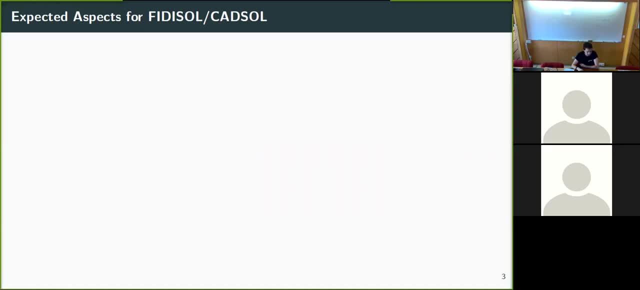 So, since it's a Newton-Raphson method, there are some aspects that are expected. The first one is that the system of PDEs must be written in this form, where all the equations in the system must be written. Basically, all the terms should be on the left side and should be equal to zero. 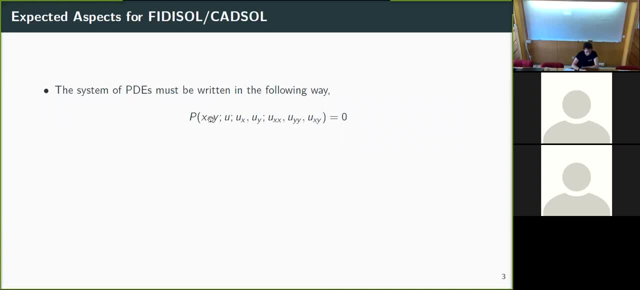 X and Y are the coordinates, basically the independent variables. U is the set of functions that we want to compute, And Ux and Uy is the first derivative of those functions and these three are the second derivatives. Then we also must provide the Jacobian for all the functions. 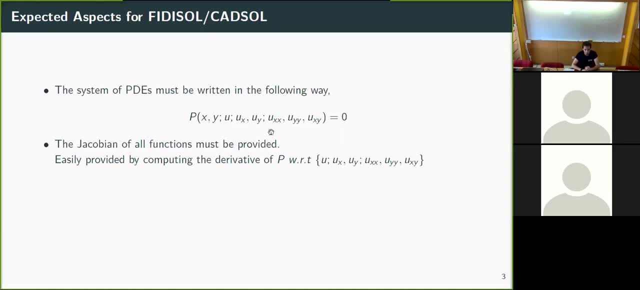 So this can be easily computed by the derivative of P with respect to all the functions, And also a good initial guess must be provided And finally, you can also provide all You have, to provide the boundary conditions in order to solve the PDE. 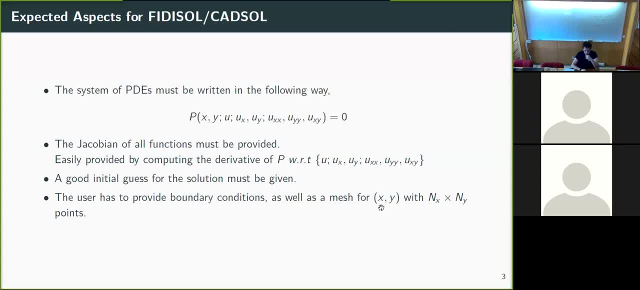 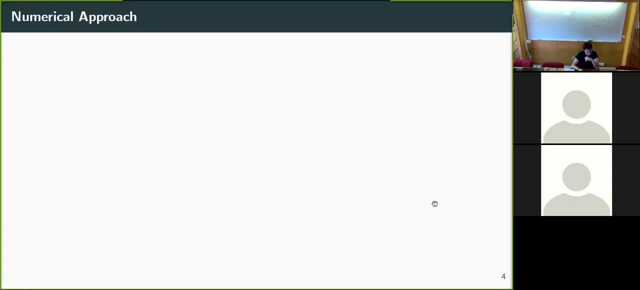 and as well as a match for, in this case, for our case, a match for the independent variables with an X and an Y points. So how does the solver really work? You start with the initial guess for U1.. That does not solve the system of PDEs. 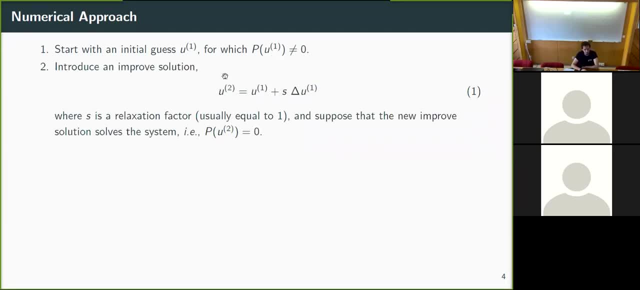 Then you introduce an improved solution in such a way where we have the initial solution plus some difference. So here X is just a relaxing factor, which usually is equal to one, And then we have some delta, which is basically just a difference. 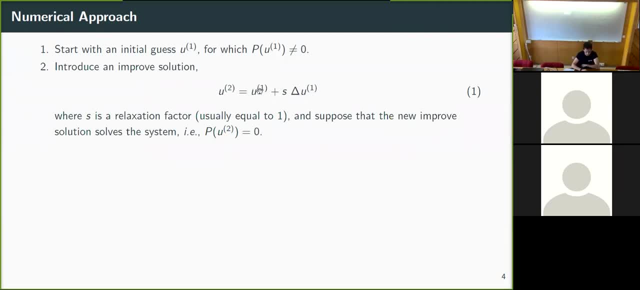 from the initial solution. Then we also say or impose, that this new solution solves the system of PDEs. Then you can expand this P of U2 in the small parameter delta U to first order and obtain this equation here. This equation, this we know because you know the initial guess. 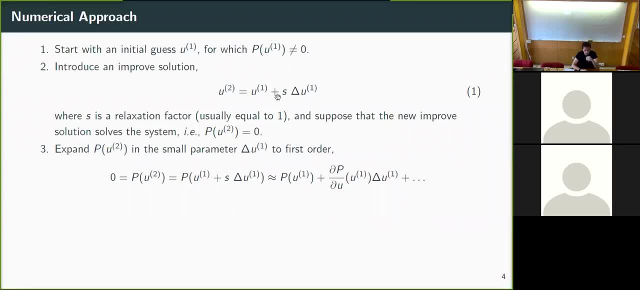 So you can just have to compute the derivative, Then you give an answer. This is the Jacobian that we must provide. So this we also know. So we can compute this delta U, And this was what I just said. 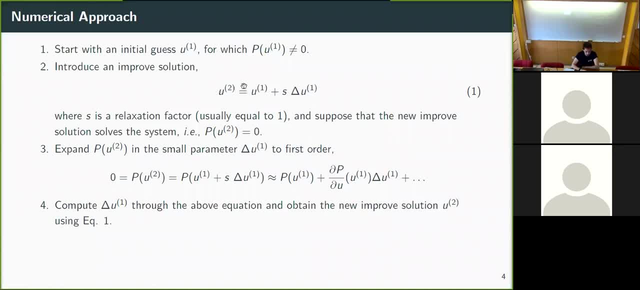 So you can use now equation one, this equation, to obtain the second or the new, improved solution. If you do this iteratively, this last three steps, until we are lower than the prescriptive data, the tolerance, we should have a good answer for the system of PDEs. 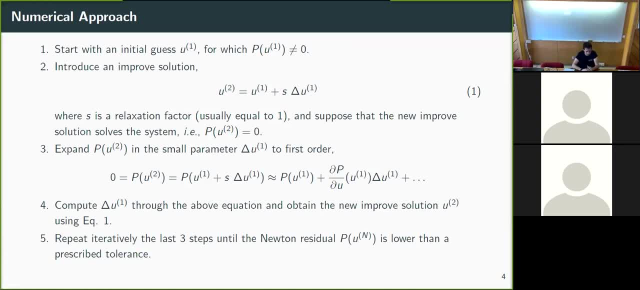 This model also came with some caveats. The first one is associated to the initial guess, So the initial guess must be close to the real solution cannot be arbitrarily far away from that. So basically, this shouldn't be very, very far from zero. 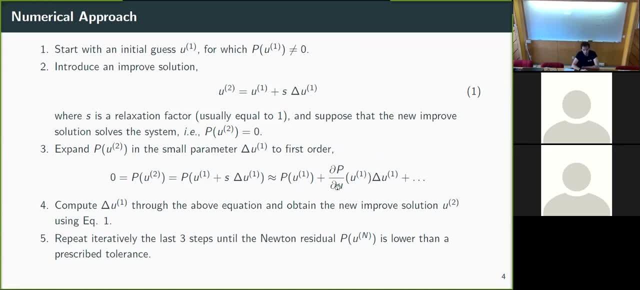 The second one is associated with this equation. It appears to be easy to solve this, But in fact what we have here is a vector. The Jacobians are matrices And this also is a vector. So in order to find delta U, we need to do inverse matrices. 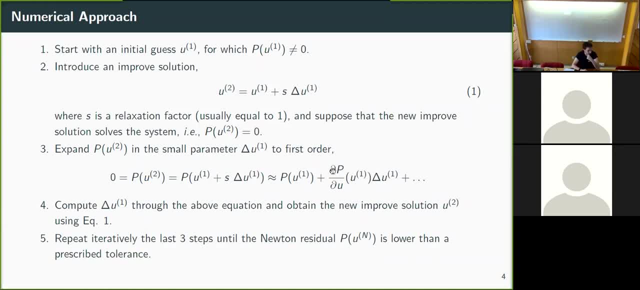 We have to solve a linear system, And this is easier said than done. But this solver also provides several linear solvers. Then you just have the users have to specify which of the linear solvers you want to use And the CAD-SOLVE will do everything for you. 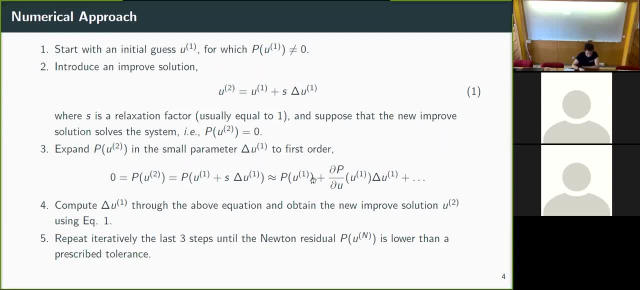 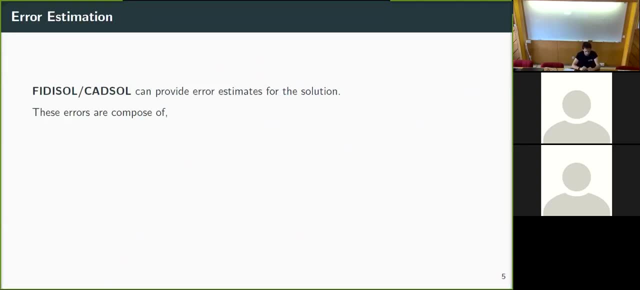 So that's a little less of a problem. So about the error exhumation, as I said, CAD-SOLVE can provide error exhumates for the solution, And these errors are composed of the Newton residuals, So the p of u of n, the last step. 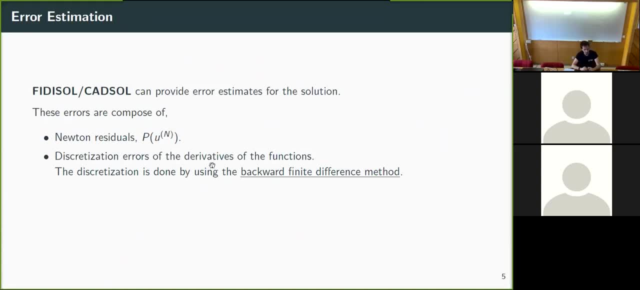 And also the discrimination errors for the derivatives of the functions. Here the solver uses a bit different. It uses a backwards finite difference method to do the discrimination And obviously when you do discrimination we always have some little error. Then you can also do our own error estimations. 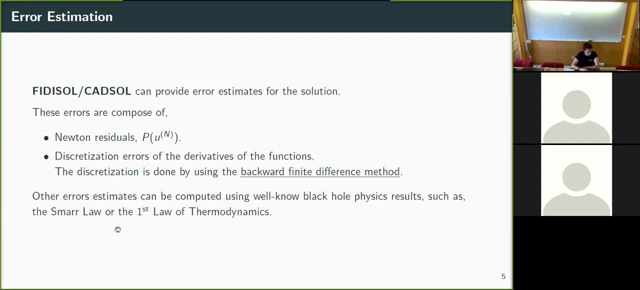 using in this case Michael physics results. It has the SMART law, the first law of thermodynamics. Now that I have explained a bit of the solver, you can now go and try to obtain a Kerr solution. So, as you know from earlier lectures, 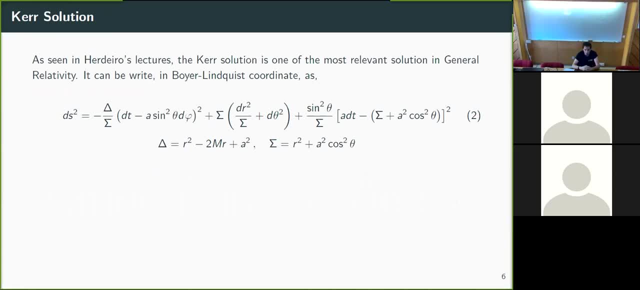 the Kerr solution is one of the most, if not the most, relevant solutions in general relativity And in boolean-linguistic coordinates. it can be written in this way: But now you can imagine that. what if Kerr never found that solution? 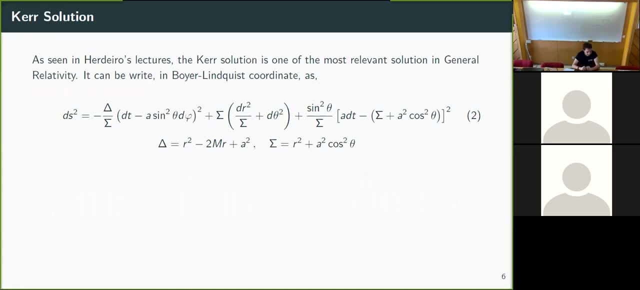 What if there wasn't some mathematician, a guy that could not find this solution? What would they have to do? You can use a numerical approach, And for that we use, obviously, the Kerr solver- Sorry, the CatSolve. 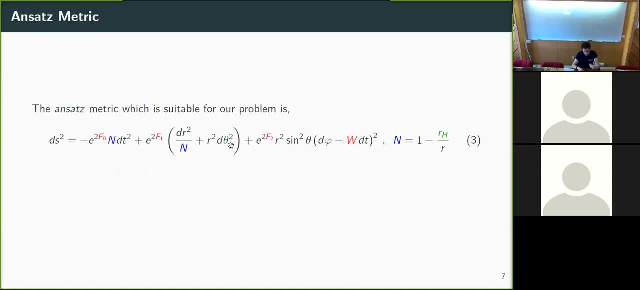 So in order to do this, you first have to impose or have to introduce an exact matrix. So here we use this type of ansatz. So here I have some colors, just to try to remember which is which. So in red we have the exact functions. 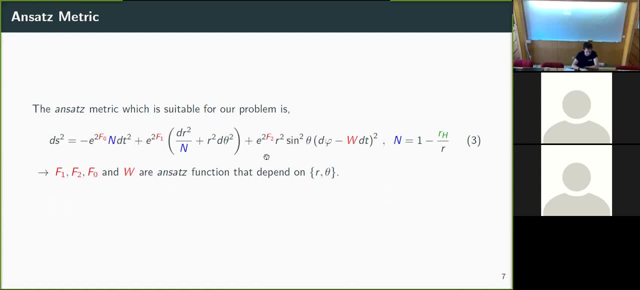 So F0,, F1,, F2, and W In blue we have some function that we define. In this case we have this n function. we define here as 1 over R, H over R, And then in green we have in this case 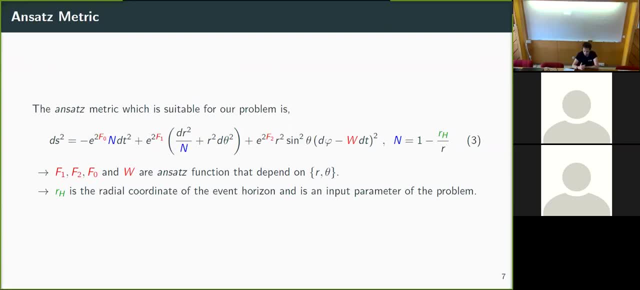 the radial coordinate of the event horizon, which is an input parameter of the problem. So if anything is written, it's the input parameter of the problem. Then well, this, although it doesn't seem the Kerr solution, can be also written: 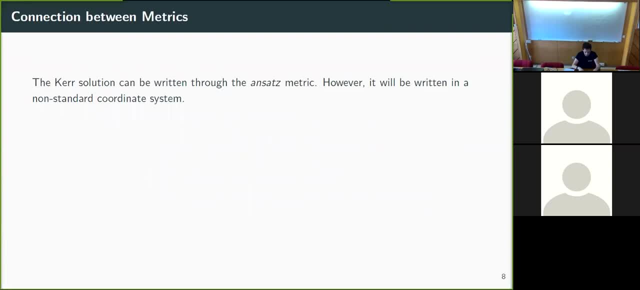 on that specific way as an exact matrix, But it will be written in the non-standard coordinate system And for that you can relate the boolean linguist coordinates with this new system with this expression. So here R and big R and big RH. 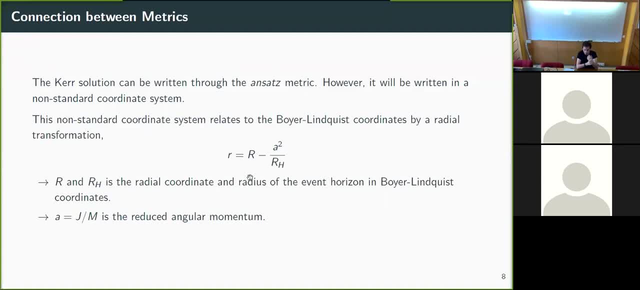 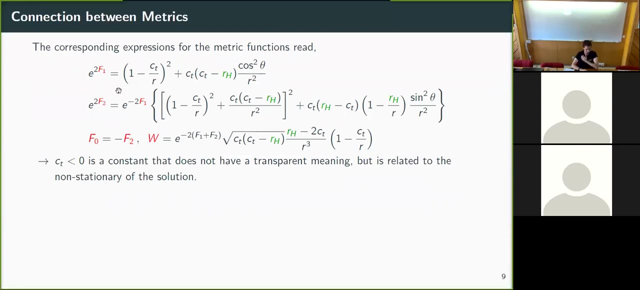 are the radial coordinates and the radial of the event horizon in boolean linguist coordinates. And this A here is just the reduced angle momentum, So you can then write the f functions in terms of the Kerr metric quantities. It's a bit confusing, a bit complicated. 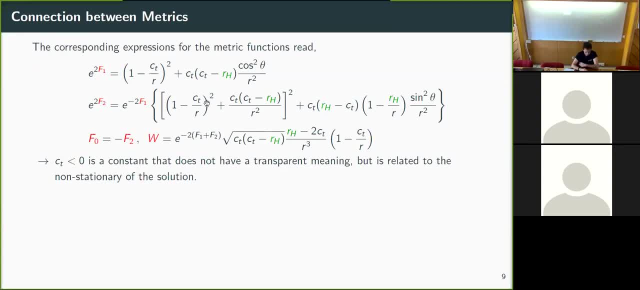 but you can do that. So here we have again RH, the radial coordinate of the event horizon, And also I have here this Cp, which must be negative, And it's a constant. so it's a constant, and it's a constant, so it's a constant. 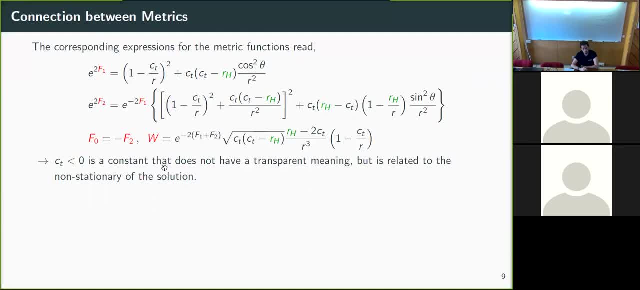 and it's a constant, and it's a constant that doesn't have a transparent meaning. But if you look at the case in which Ct is equal to zero, this will be apparently related with the non-stationarity of the solution. This can be further verified. 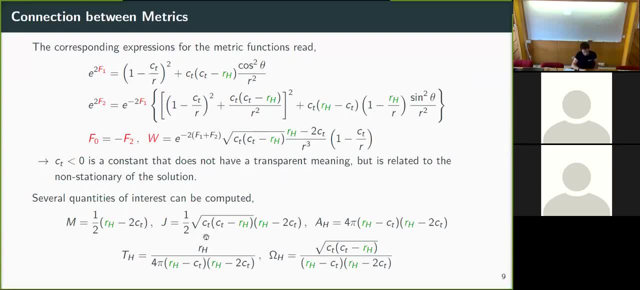 when you compute the physical quantities. So here we have the angle momentum, and if you put Ct to zero, the angle momentum is zero and the horizon's angle of velocity is also zero. So you can have a sense what this Ct is. 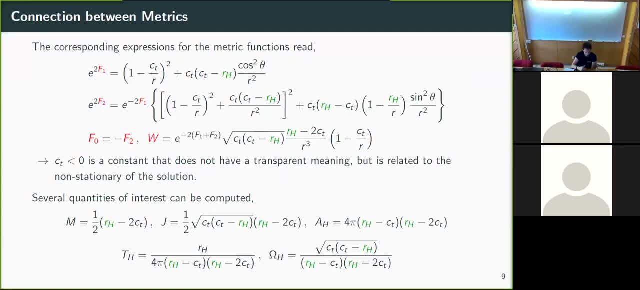 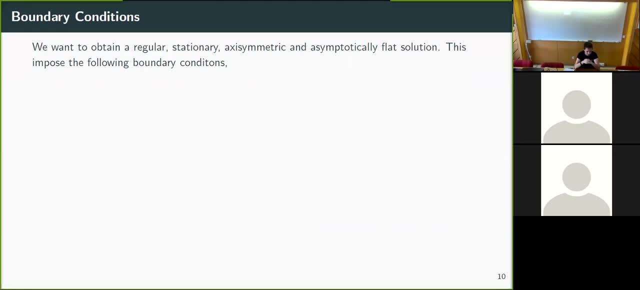 but from outside of that it's not very, very meaningful. So now that we have a metric, we have to impose boundary conditions. Since we want a regular, stationary, azimuth, metric and asymptotically flat solution. this will impose some restrictions for the functions in the boundary conditions. 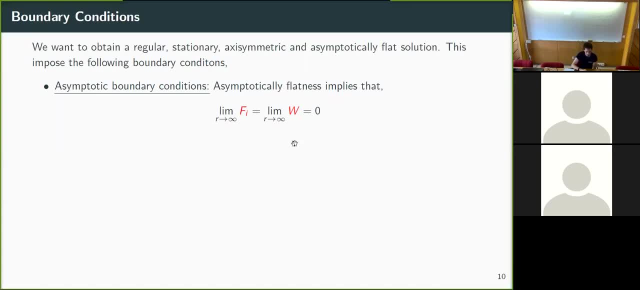 For the asymptotic boundary conditions, it's quite easy to see that since we want asymptotically flatness, all the f functions and the w function must be zero, must go to zero. Then for the axi boundary conditions, axial symmetry and regularity implies that on the plows 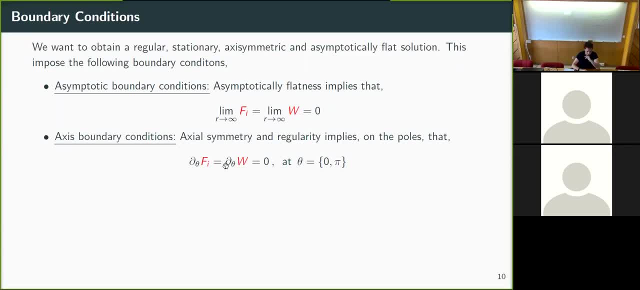 the derivative of the f function and the w function in order to theta must be equal to zero. Also, since we don't want to have conical singularities, there is the f1 must be equal to f2 when we are on the plows. 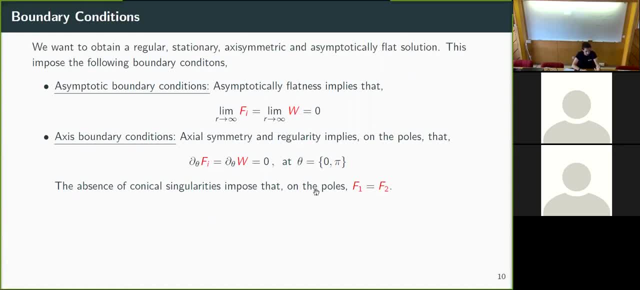 We don't impose this as a boundary condition, but we'll use this result as a test for the numerics. Then, since we have also a symmetry related to the equatorial plane, we can compute everything just in a region from theta goes to zero to pi over two. 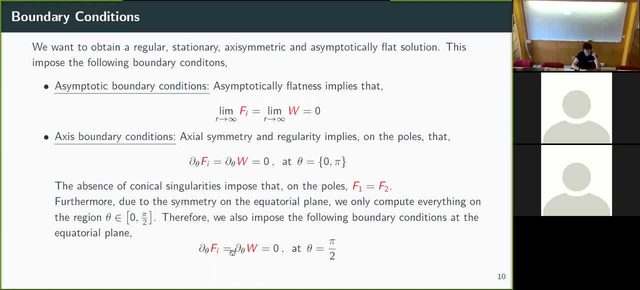 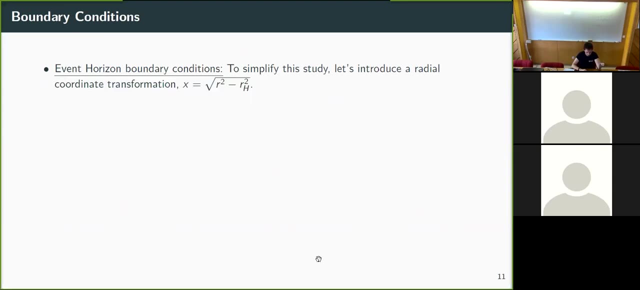 If we do this, then we also have to impose that on the equatorial plane these derivatives of the f function and the w function also must go to zero on the equatorial plane. Then we just have to then go to the event horizon. boundary conditions. 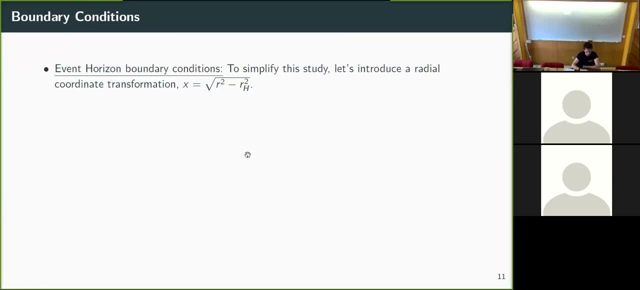 And to do this it's easier to do coordinate transformation of this type. This way, when we are at the event horizon, x equals to zero- We can do a series expansion of the function and we obtain these results. And here we see that the w function. 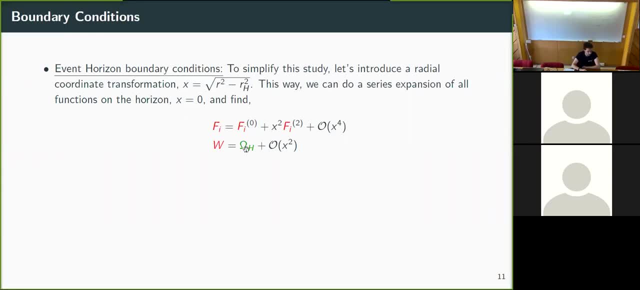 must be equal to omega h. This is a constant and, as you see, it's green, so it's an input parameter of the problem, And this can be understood as the angle velocity of the event horizon. Then, so, with this expansion, 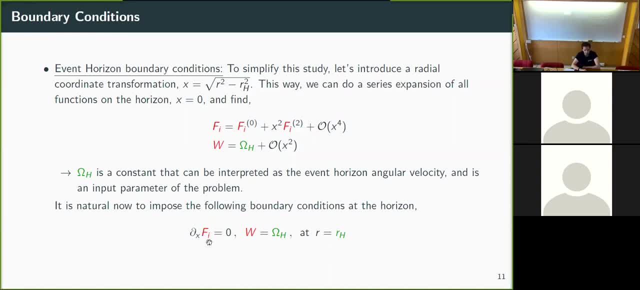 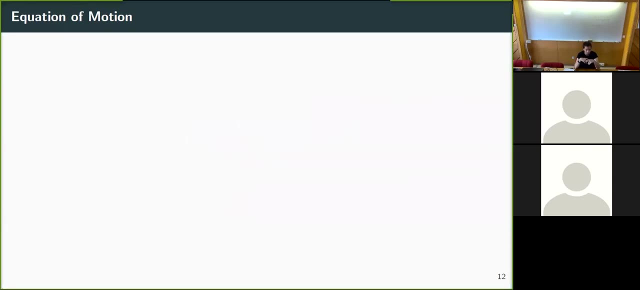 it's quite natural to impose that the derivatives of the f functions must be equal to zero and that the w function must be equal to the horizon: tangential velocity at the event horizon. Now that we have the metric and the boundary conditions, now we just need the equations. 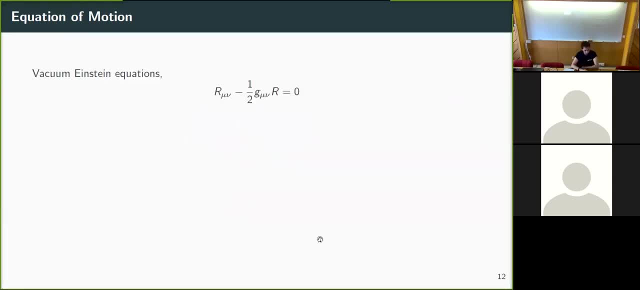 equations of motion. These are computed through the Einstein equations, so in this case the Bakken-Einstein equations. So to do this and to be easier for analysis afterwards, we'll keep the radial coordinate that I show in the last slide. 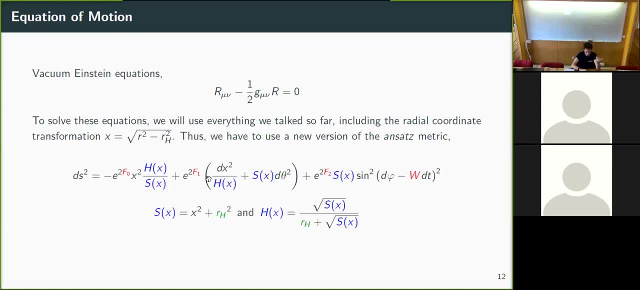 So here we have to rewrite the ansatz in this way, in this new way, since we impose a new radial coordinate, And, if you want, you can try to prove that this h function and s function are equal to this. So I can leave you as exercise, if you want. 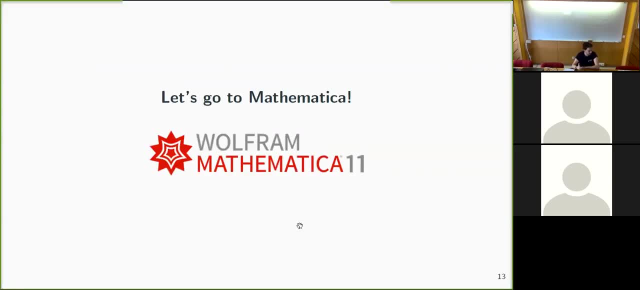 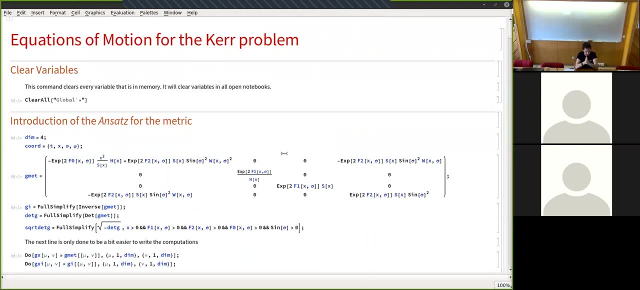 So, now that we have all of this, you can go to Mathematica and use it to obtain everything that you want. So for that, here I have the first notebook, which is the equations, equations of motion underscore curve. So here we start by this first line. 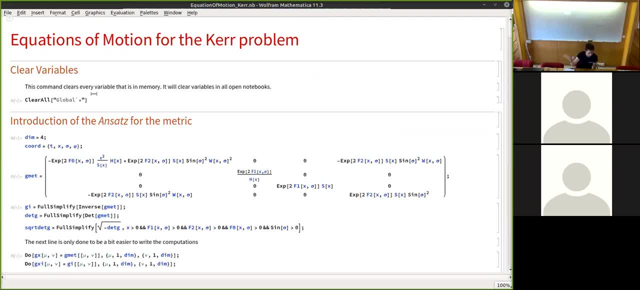 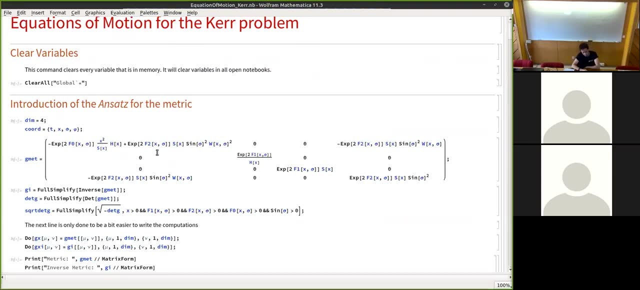 is just to clean all the variables that can also be used by other notebooks. So first we introduce the number of dimensions and the coordinates and the metric. With this you can compute the inverse metric, the determinants and the square root of minus the determinant. 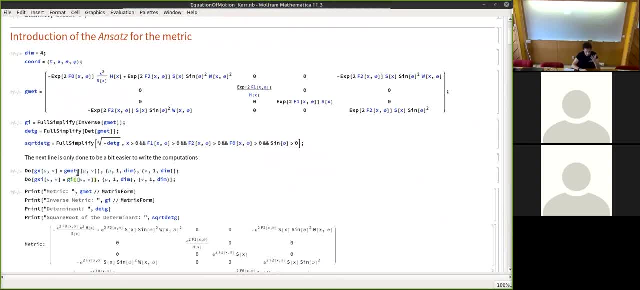 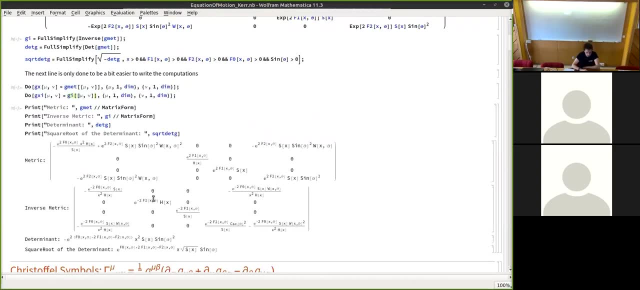 Here these two lines are just to simplify a bit the notation. It's not very tricky or very You don't have to do this. Then here just some prints to see some quantities. So now we have to compute the Christoffel symbols. 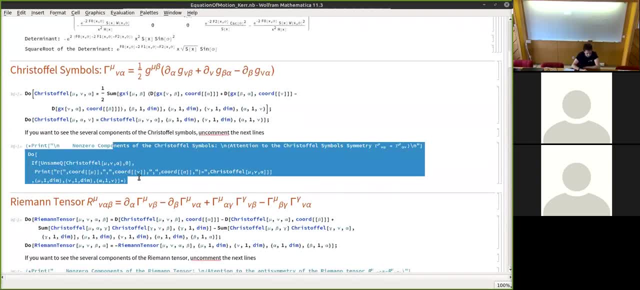 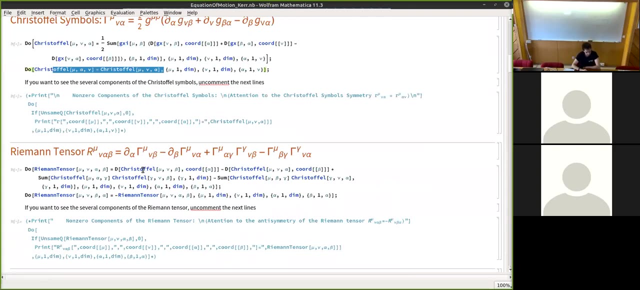 So we can do this. This line here is just to print the non-zero components of the Christoffel symbols. Also, I use the symmetries of the quantities to be a bit faster. Then with the Christoffel symbols we can compute the Riemann tensor. 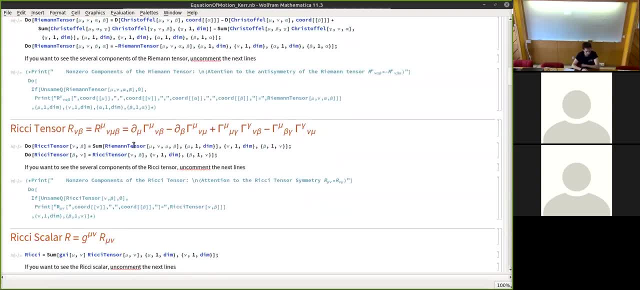 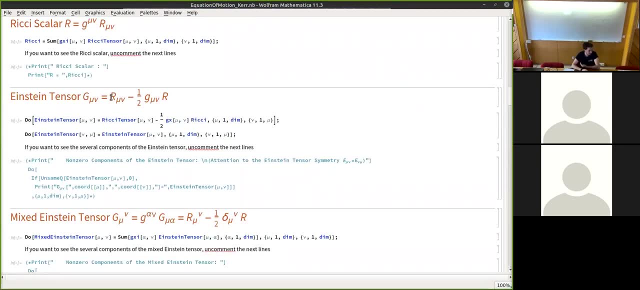 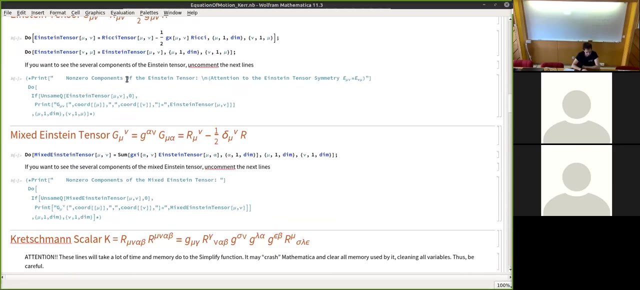 And with that you can go obtain the Ricci tensor and finally the Ricci scalar. So you have now the Einstein tensor, which in this case is the equations of motion You can compute. And here we, instead of using the covariant version of form of Einstein tensor, 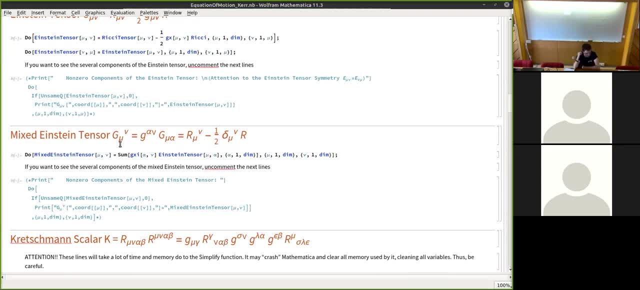 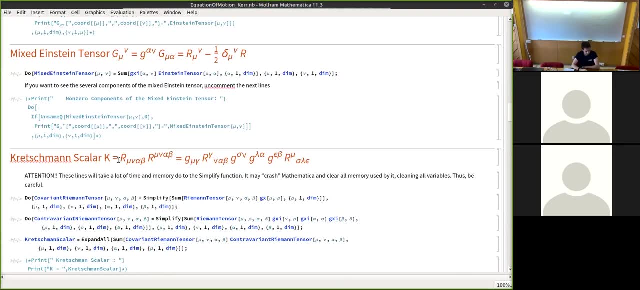 we use the mix, So one of these is covariant, the other is a contravariant. Then you can also compute the Kretschmann scalar. This is not an important step, but it's useful to see if, when you obtain the solution. 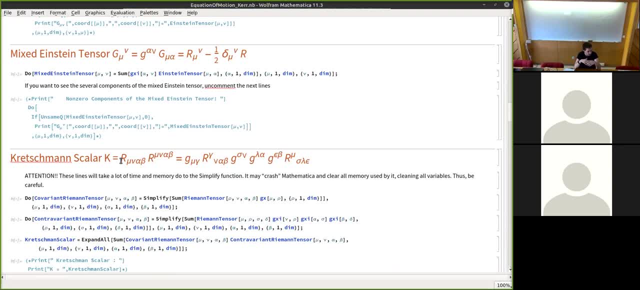 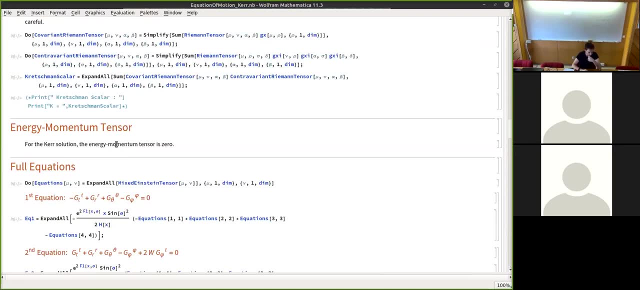 if the spacetime is smooth everywhere, if there is no divergence. if there is no divergence, Then here I have a part for the energy moment tensor, since we want the Kretsch solution, that is equal to zero, so not a very important step. 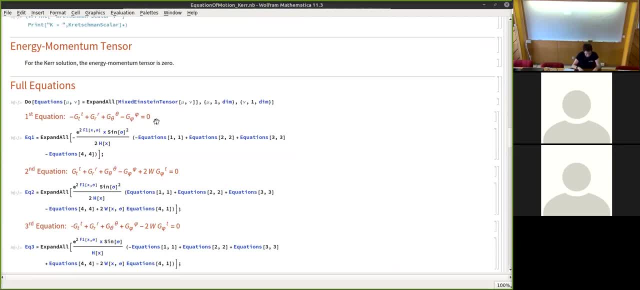 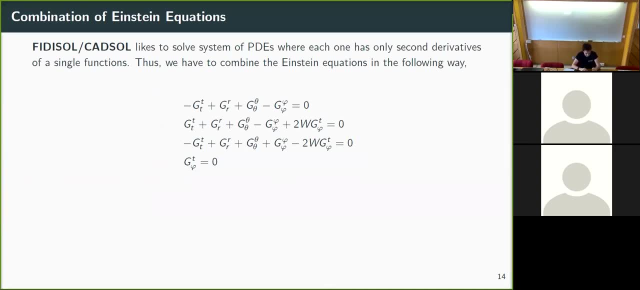 Then you have basically the full equation. So here, instead of using all the equations as they are, you will do a combination of the Einstein equations. This is done because Katzoff likes to have all the PDEs written as having only one function. 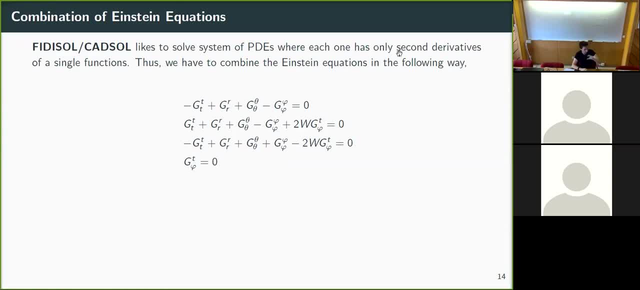 with second derivatives. So he wants, for example, for the first equation he wants that to have only the second derivatives of the f1 function, for example, and the second one for the f2, and the third for the f0,. 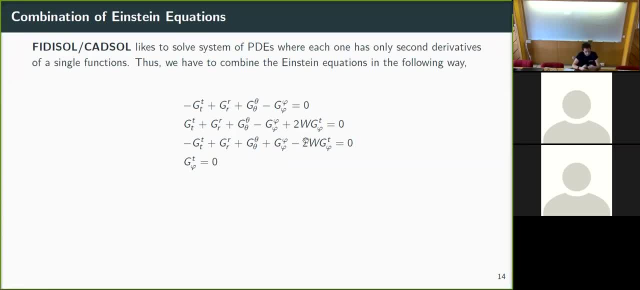 and the fourth for w. So you have to do a combination of these Einstein equations. you can do this in this way. that will give you exactly what Katzoff wants. Then you also have another two equations that will be used as constraints. They will not be solved by the solver. 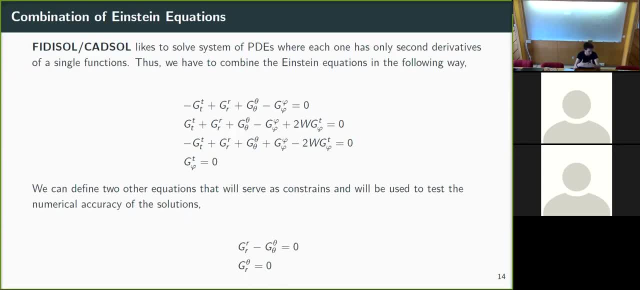 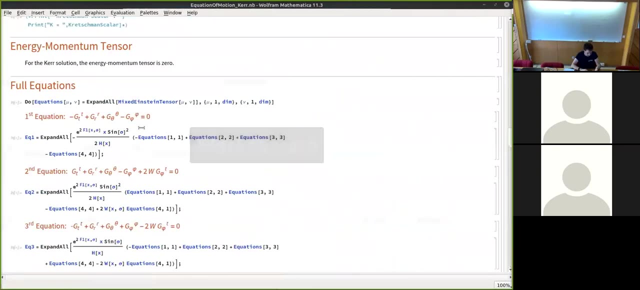 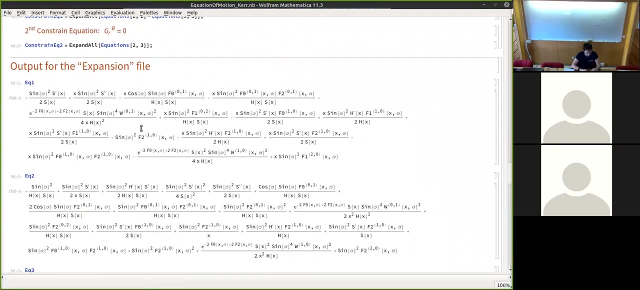 they will just be computed with the solution that you obtained and will be basically just to see if the solver obtained a good solution, if the, if everything went well. So here I do exactly that. so it's not very interesting, but then you can do the print. 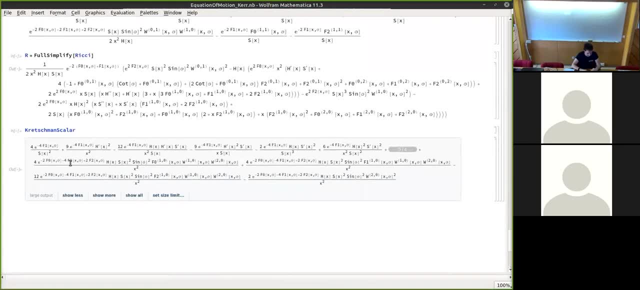 just to see how the functions are Here. as you can see, the Krashman scalar has a lot of terms. Then with the equations of motion, you can now do a series of expansions of them in the boundary condition or in the boundaries. 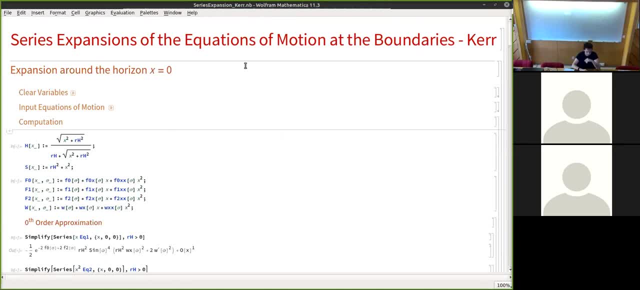 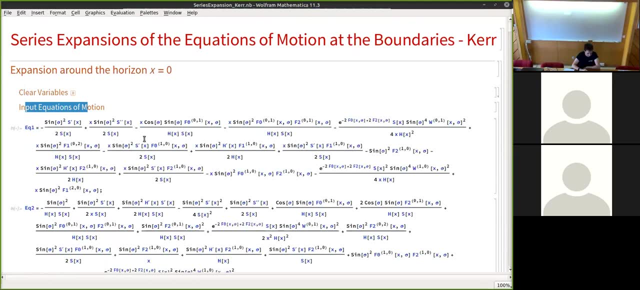 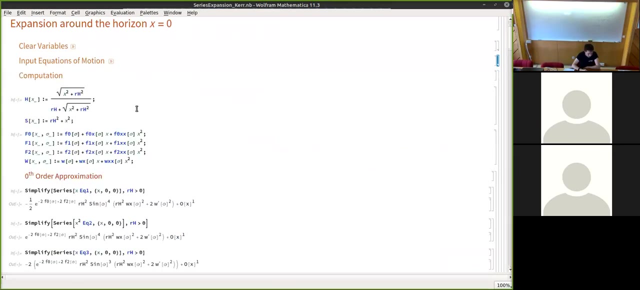 For that we have the series expansion, underscore, curve notebook. So here, first I clean the variables again and input the equations of motion, as you can see. Sorry, Here And now for the expansion of on the horizon, where x equals to zero. 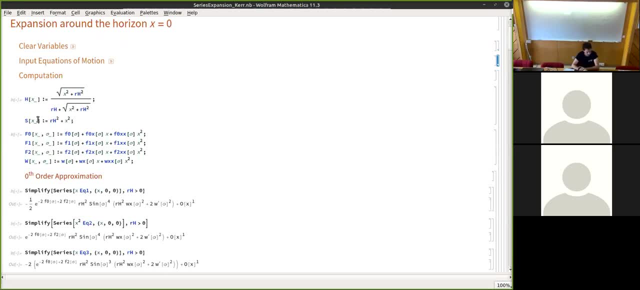 we have to redefine again or introduce again the h function and the s function, since they depend on x, And then we can do a power series of the functions in x, as you can see, So doing the first-ordering approximation. 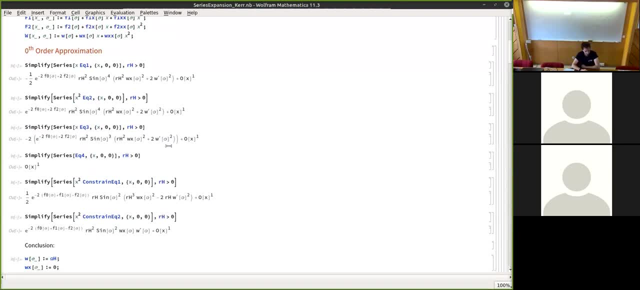 you obtain these results. Since each one of the equations must be equal to zeros, then these results also must be equal to zero. So for example, for example, from this equation, you see that for this to be zero, either wx or the derivative of w. 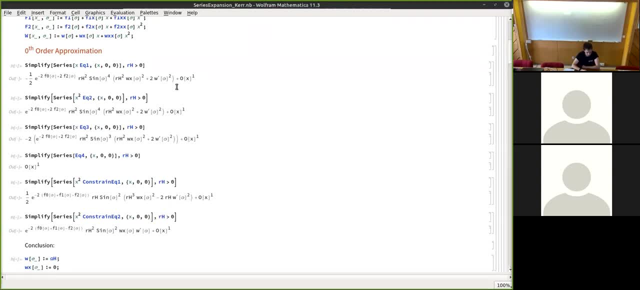 must be equal to zero. And if you look to the other, these other four equations, if one of them is equal to zero, then the other must also be equal to zero. So we conclude that wx must be equal to zero and the derivative of w must be equal to zero. 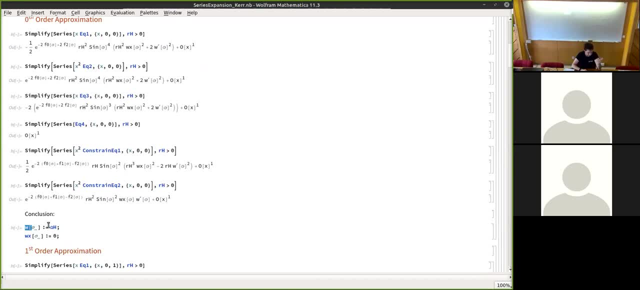 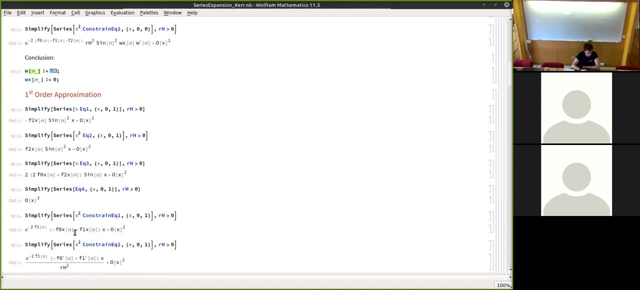 Therefore the w must be equal to a constant, And here you say that the constant is omega h. Then, going for the first-ordering approximation, we do the same, And from these two equations we see that f2x must be equal to zero. 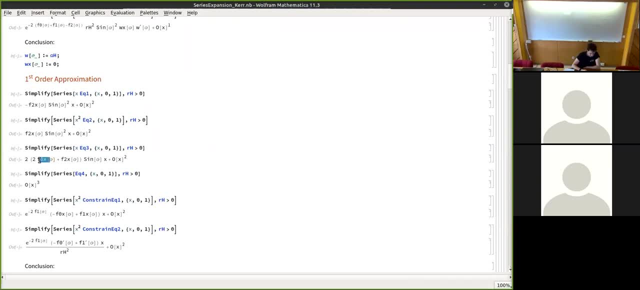 This implies that on the third equation f0, x must also go to zero. And finally the fifth equation. we see that f1 also, f1x also must go to zero. Then this last equation basically says that the derivatives of f0. 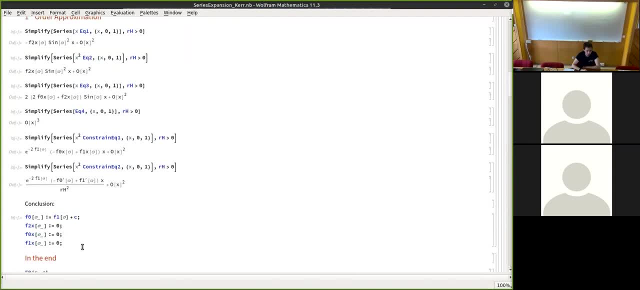 must be equal to the derivative of f1. This includes this implies that f0 must be equal to f1 plus a constant. This is related to the fact that on the horizon, the Hawking temperature must be a constant. This is basically related to this result. 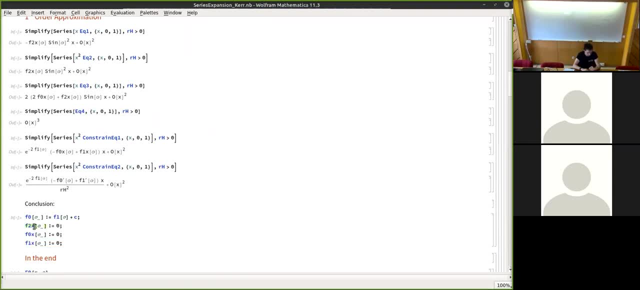 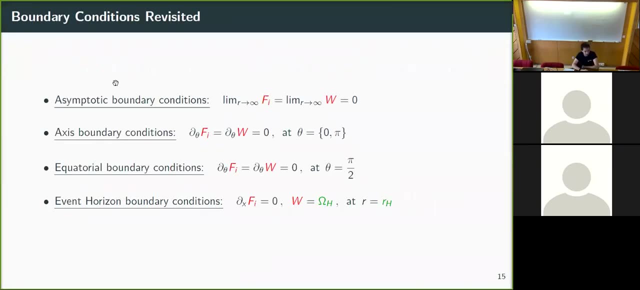 So we also impose, from what you see before, that the f functions x must be equal to zero. This is exactly what we all see for the monocreditions at the event horizon. So the derivatives of the f function must be equal to zero. 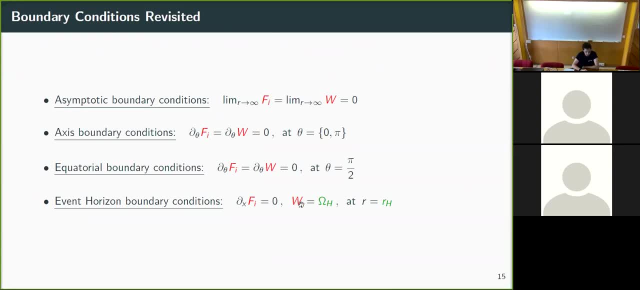 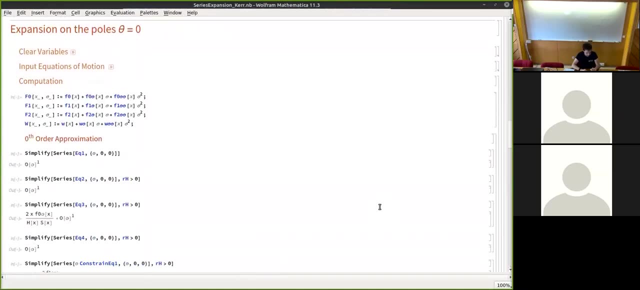 and the h function must be equal to omega h At the event horizon. If you do the same for the poles on the pole, you can do it. do exactly the same, but now the power expansion is on theta instead of x. 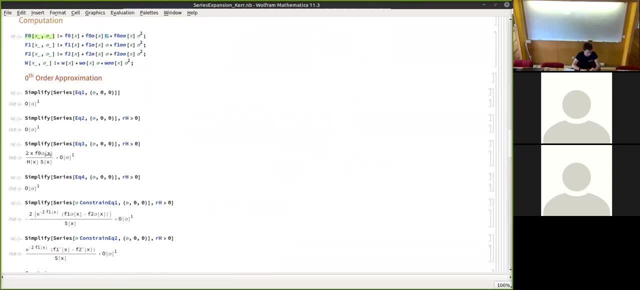 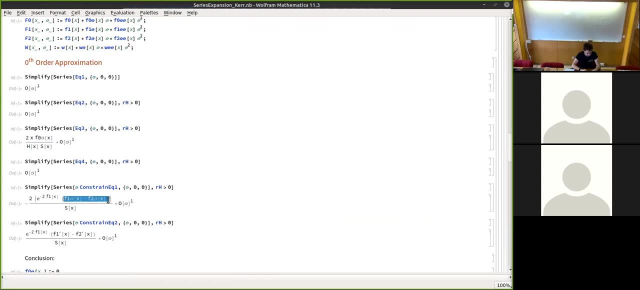 And if you do as I said, they're exactly the same. So here we see that f0 theta must be equal to zero. Here we see that f1 theta must be equal to f2 theta, And here we see that f1,. 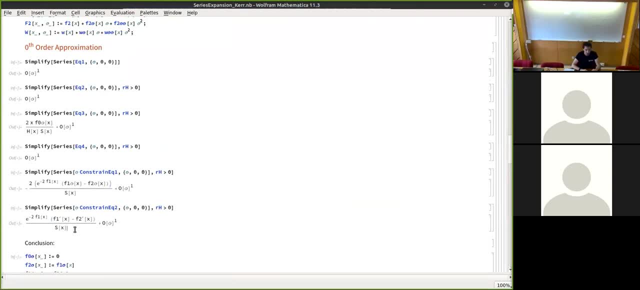 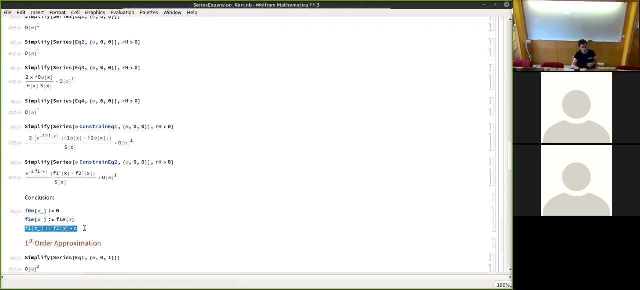 the derivative of x1 must be equal to the derivative of x2.. So we write this. So this result: here: f1 must be equal to f2, plus a constant is associated to the conical singularities. In fact, this constant must be equal to zero. 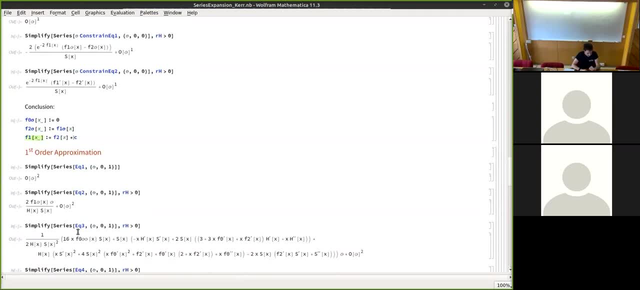 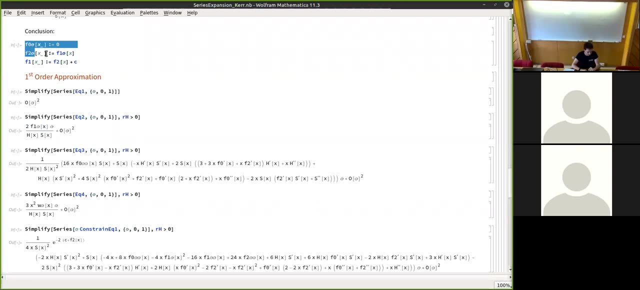 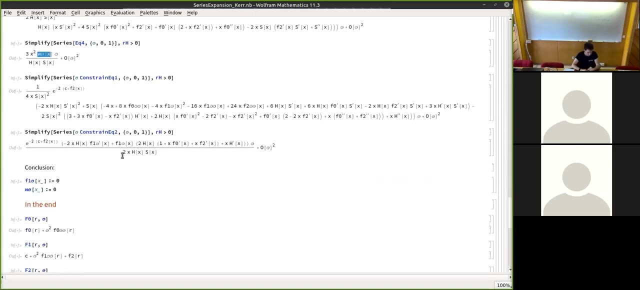 because of that. Then, going for the first ordinate approximation Here, we see that f1 theta must be equal to zero, So f2 will always be equal to zero. And we see that delta theta must also go to zero. So we say that. 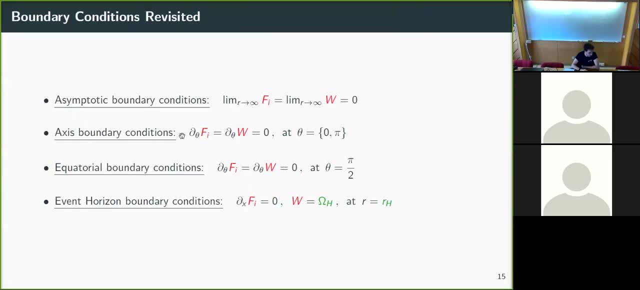 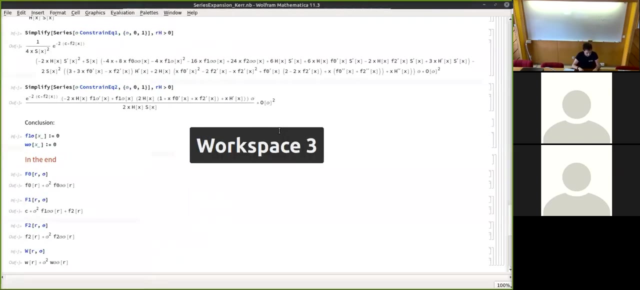 And again, this is exactly the same result that we impose for the poles: that the derivatives of f1, f2, and f0 and the derivative of w must be equal to zero. So now that we motivated a bit more why we choose this boundary conditions. 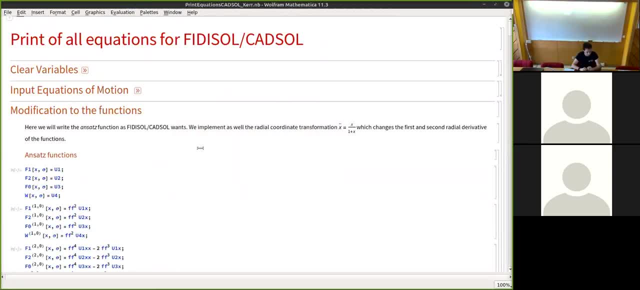 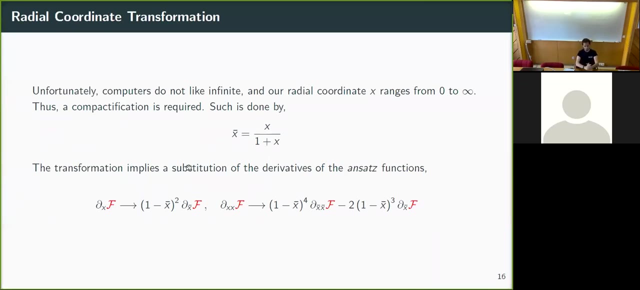 we can go and print everything that we obtained so far in the format, in the Fortran form, so that we can compute or copy everything to Fortran file. But before we do that, the radial coordinate that we use goes from zero to infinity. But computers don't like. 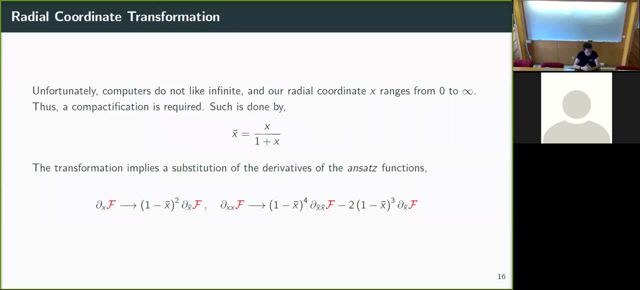 very much infinity quantities. So it's useful to use, to impose a compactification, And one way of doing this is basically doing this coordinate transformation. And since we do this coordinate transformation, the derivatives will also change and will change in these factors. So on the mathematical file. 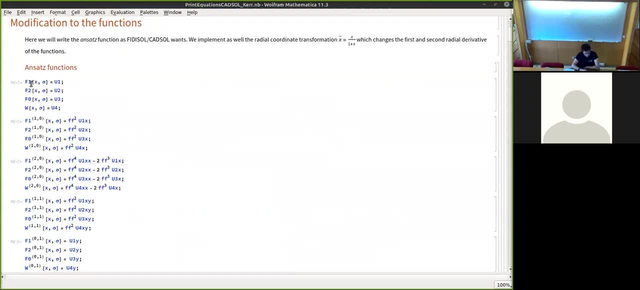 you can say that. So here we say that f1, f2, f0, w are equal to u1, u2, u3, and u4.. And the derivative, or the first derivative in order to x or to the radial coordinate. 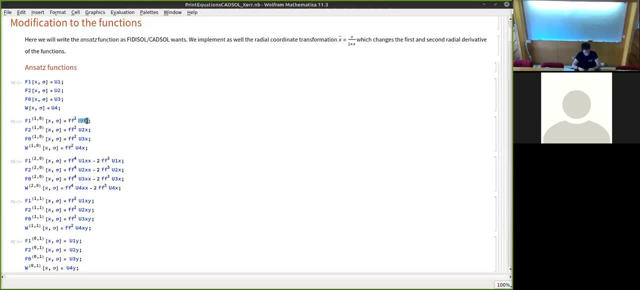 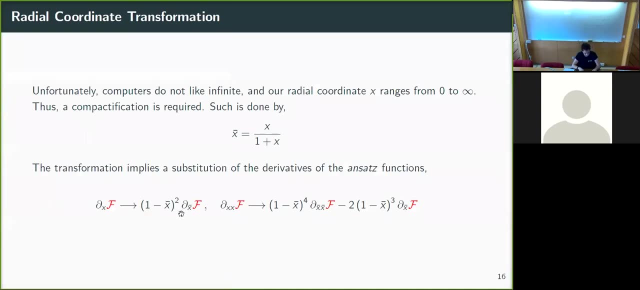 will be this: ff squared times. the derivative which is, if you look to this, is exactly ff- is one over x bar. Doing the same for the second derivatives. This is exactly the same. You can do everything. And now we have here: 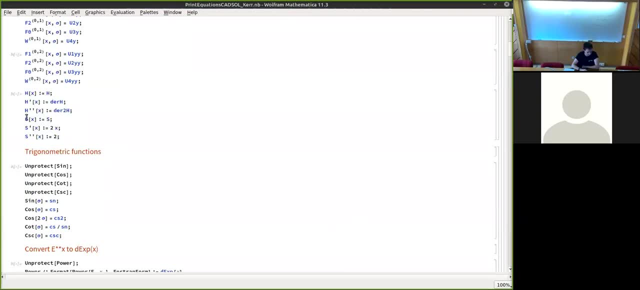 we write the h function and the x function. So here we just say that is equal to this name, And on the Fortran file we'll specify the expression. It's a bit long, so that's why we do this here And then on the Fortran file. 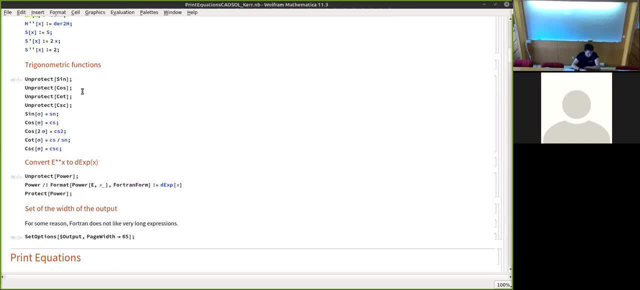 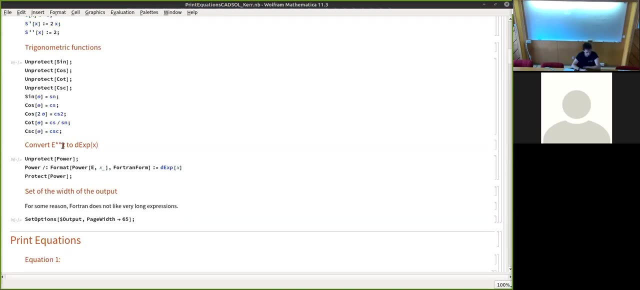 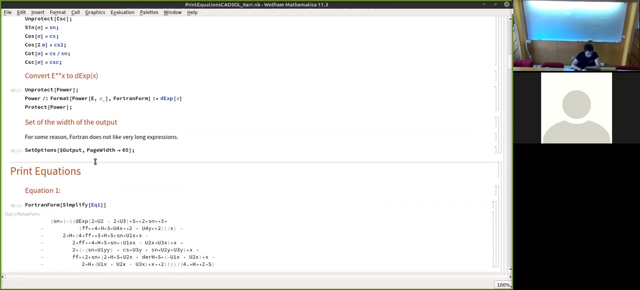 we specify the function Here. we just rename the mathematical functions for the sine cosine and the others to be a bit easier when we write everything on the Fortran file. And we also do the same for the explanation. Now, for some apparent reason, 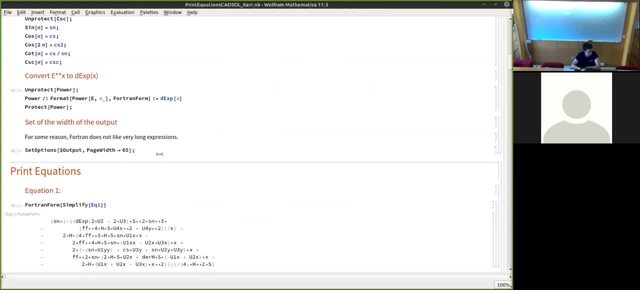 Fortran doesn't like very long expressions, So it doesn't like the expression to be in just one line. So we have to basically shrink the width of the page to some value, so a bit smaller. So that's when you print everything. 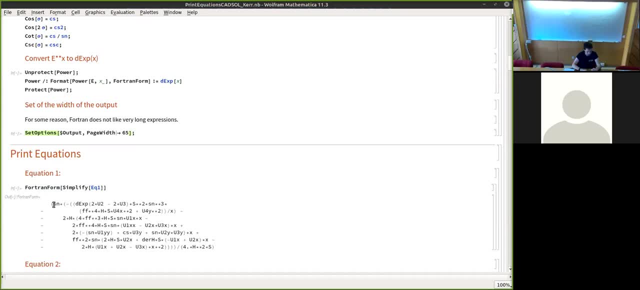 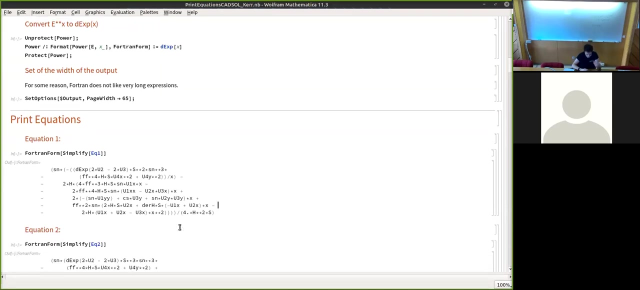 for example, the first equation of motion in Fortran form, you get something like this: No, I know, I know there should be a reason, but I didn't know which was. But yeah, it makes sense, So you can do the print. 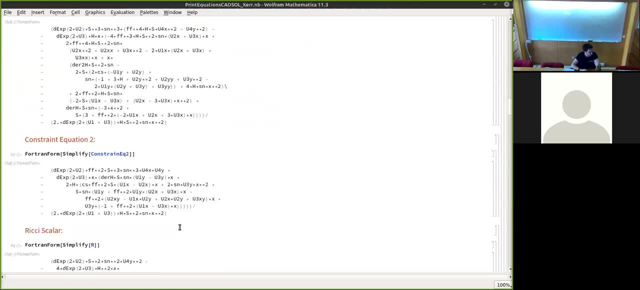 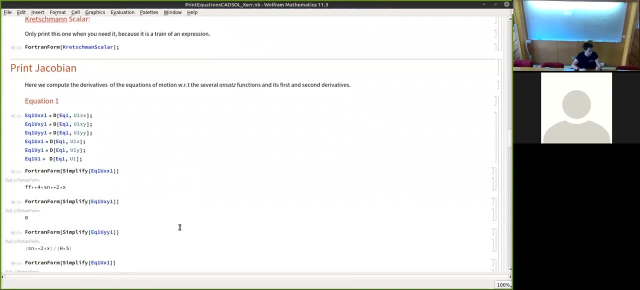 and then we have just to copy this to a Fortran file, as I will show you next. And just to finalize this part, as I said, you need the Jacobian, So you need to do the derivatives of each equation in order to each function. 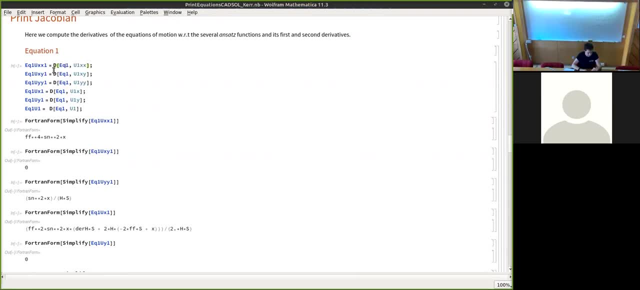 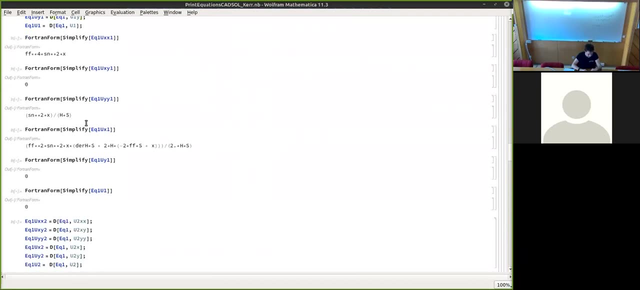 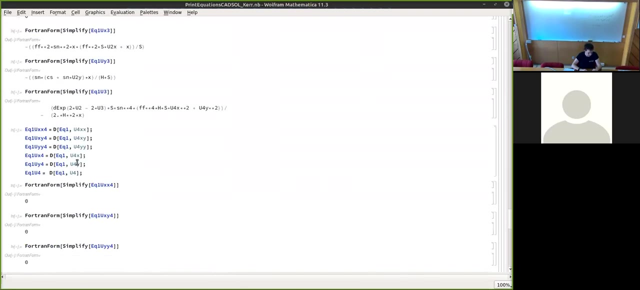 and their first, second derivatives. So here for the equation one. we do the derivatives with respect to the function one in the derivatives. So get some results. then for the function two, F2, then for the third function and then for the fourth. 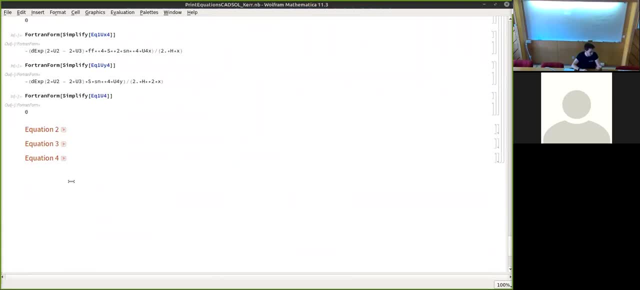 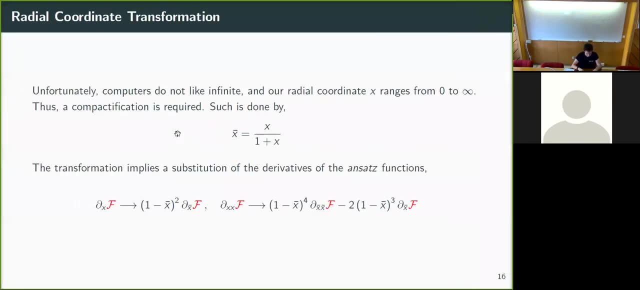 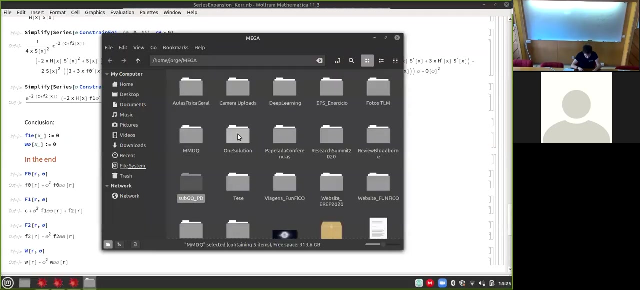 And we have to repeat this for the remaining three equations. So, as you can see, that will be a lot of small expression. Now, with this done, you can go to- let me just go there, Not here. You can go and print everything. 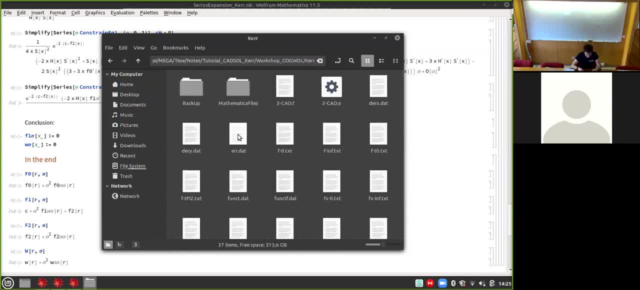 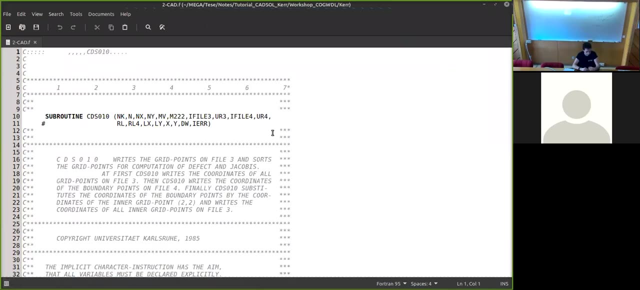 for the Fortran file. So the first one is this: 2C2CADF, And this is basically the brain of the solver. So within this file there are several subroutines which are appropriate for some type of problem that you have. 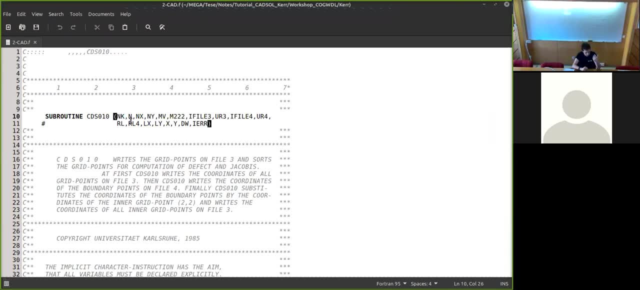 So in our case, we want to save or want to solve analytic solver problem, So we will use some specific routine, But if, for example, if you want to solve parabolic problem, you use a different subroutine, Since this file is the brain. 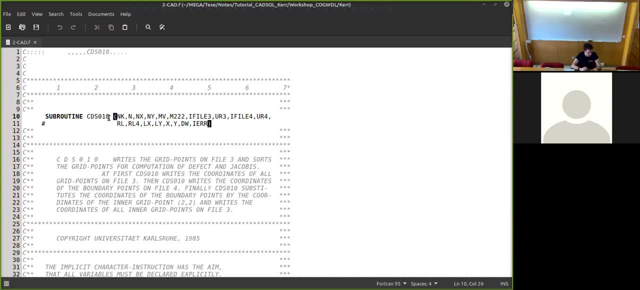 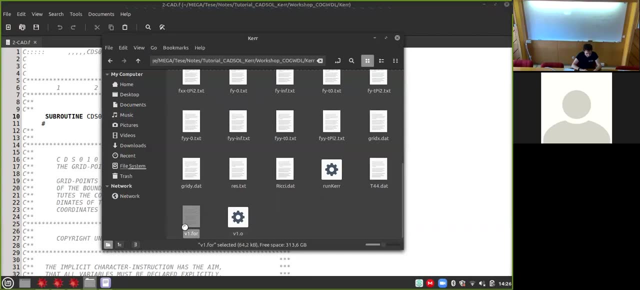 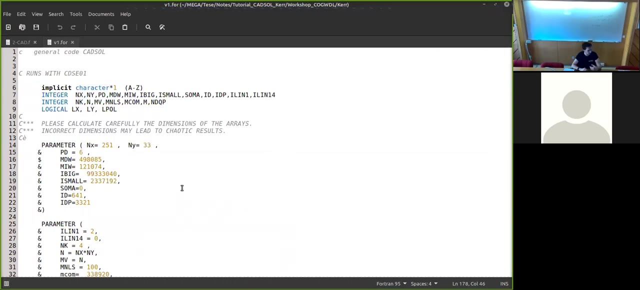 of the operation. you should not mess with it, Even if it is don't change anything. Then we have the file that we will change And here is where everything, everything that you compute so far, will put everything there. So you start by defining. 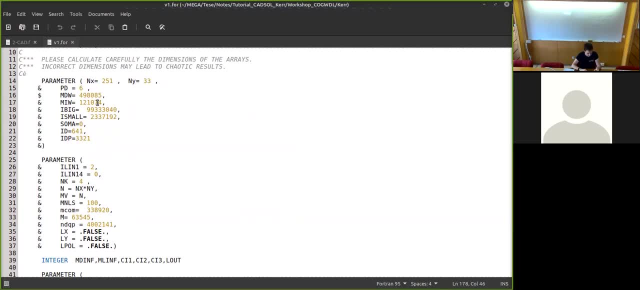 some parameters for the solver. There are a lot of them. I will just mention some which are a bit more important. So the first one, or the first two ones, are the number of points in the grid for in the x-direction, in the y. 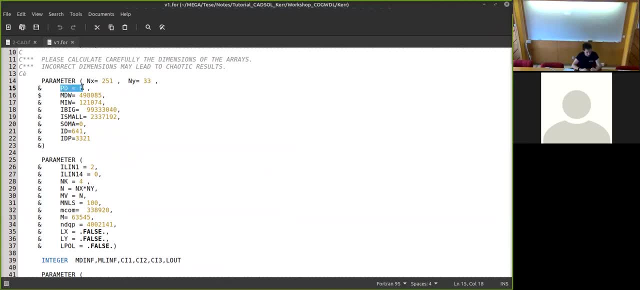 the x in the y-direction. This PD is the consistency order for the linear solver. Then this- I am in one- is then the solver that you want to use. So he uses numbers to define or to specify which solver he is, Sorry. 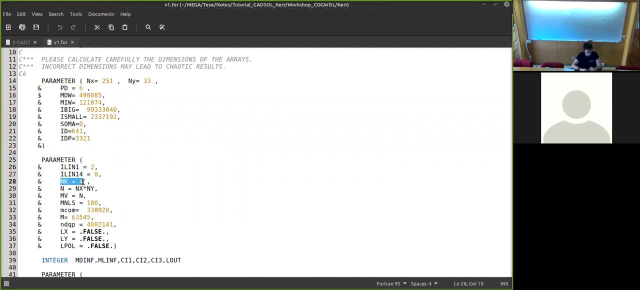 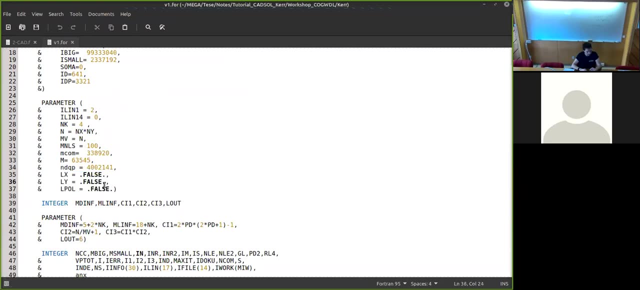 Then this NK is the number of equations that you have to solve. Then, for example, this LX, LY and pole is, if you want, or if your bonding conditions are secular, So if they repeat themselves, In this case it doesn't. 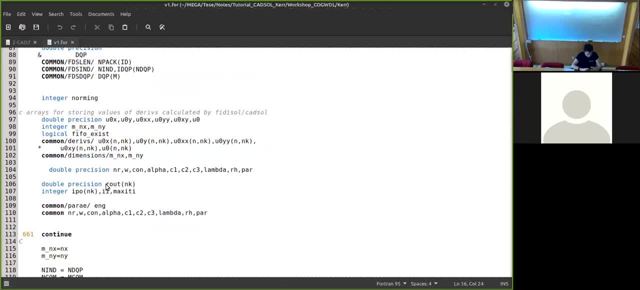 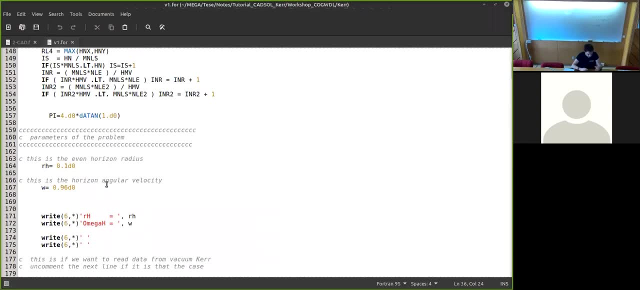 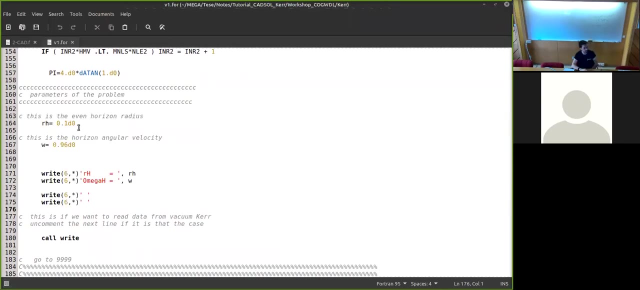 So you put as false. Then there is a lot of code for the solver. This has to do with memory and so on. It's not very, very important here. So next we have the parameters of the of the problem You have to input. what are the? 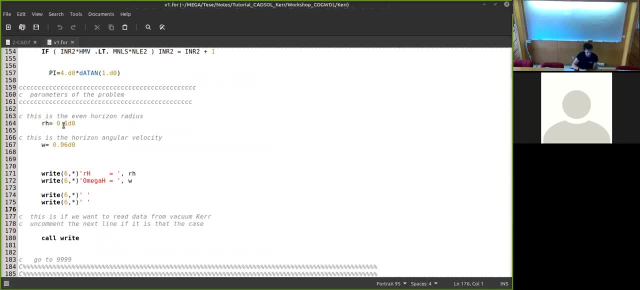 the parameters of the problem. So the one- the first one, as we saw- is event horizon And the second one is the horizon tangler velocity. Here we put these values, for example. Then there's also this subroutine, which was developed by Dr. 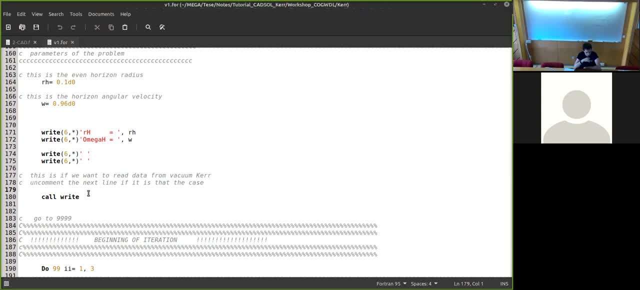 Eugene Radu, that when, in this case, since we have a curve solution, we can use as an initial guess the, the, the care solution obtained by equations that I, I saw, I show you on the presentation. But if you use mathematics, 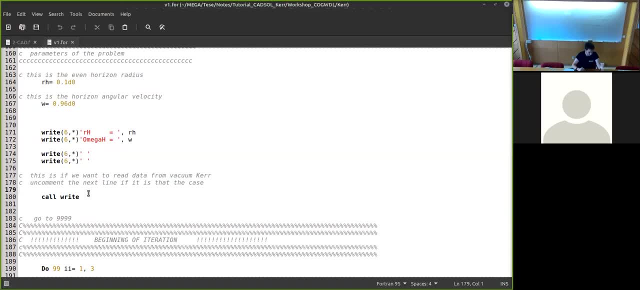 for example, to obtain what are the values of the, the F functions in the double function. Fortran doesn't like very much the way that it's written, So this function or this subroutine, what does is read those numbers, put everything as Fortran wants. 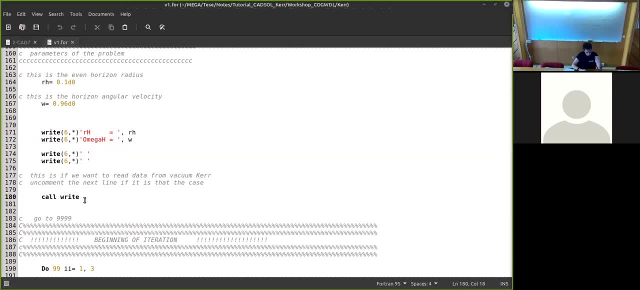 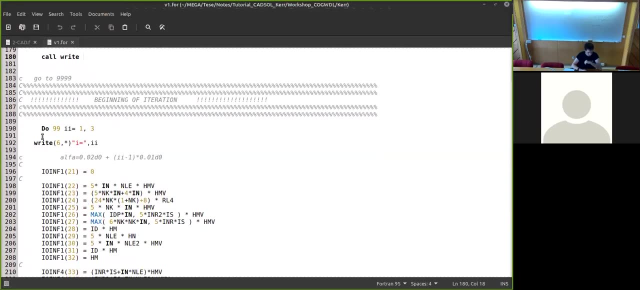 and then print again or everything. So when you use that file as the initial guess, Fortran will not have any problem with that. So here is when we begin the integration for the Newton-Hafson method. Usually use three iterations. Usually it's enough to obtain good accuracy. 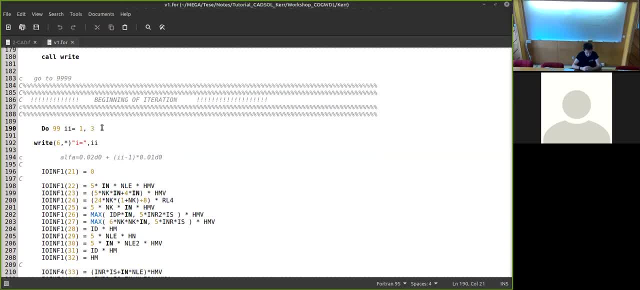 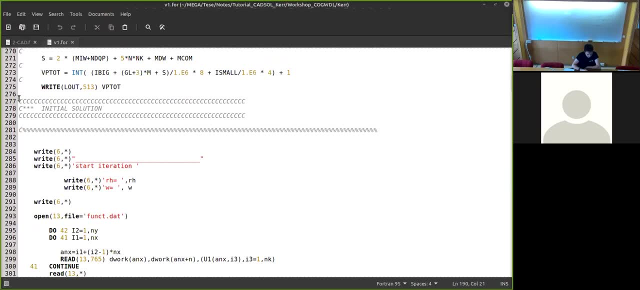 Of course, you can do more if you want, but usually three is enough. Then this is. this is some parts of the code, And here it's where we start. you go get the initial solution, which usually is on this file, on this name file. 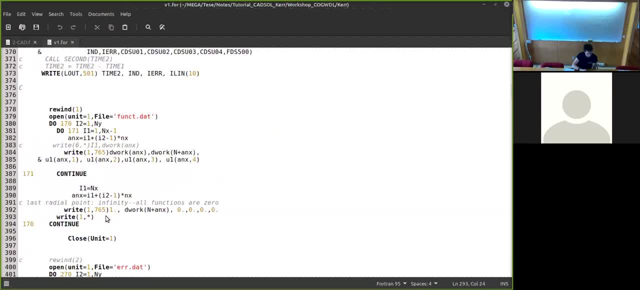 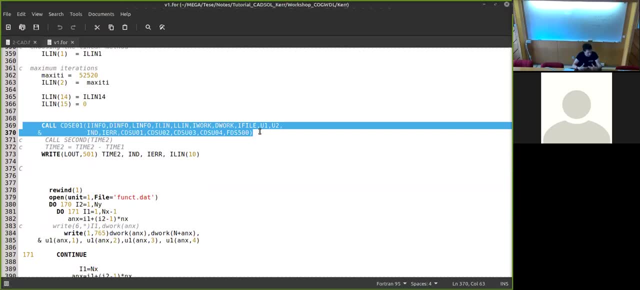 Then again a bit more code. Here is where the real code begins. So, basically, here he calls the subroutine, which is this one in particular for our code, for our case. And here is when you do the, exactly the Newton-Hafson method. 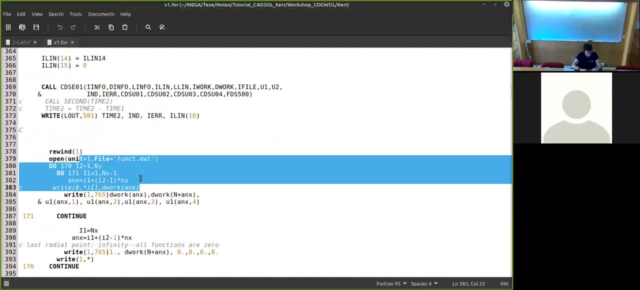 So after this, after the computer, it will print everything. So in this file we'll print the, the UNZAP functions F1,, F2,, F0, and W. You also print the errors Printed, the grids. 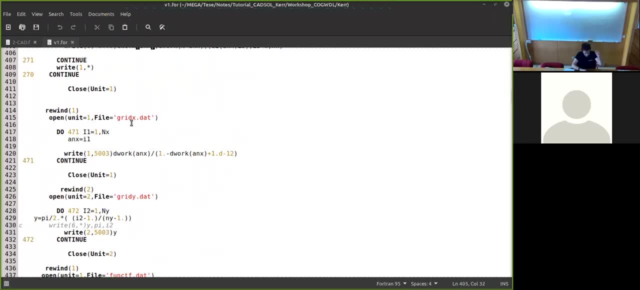 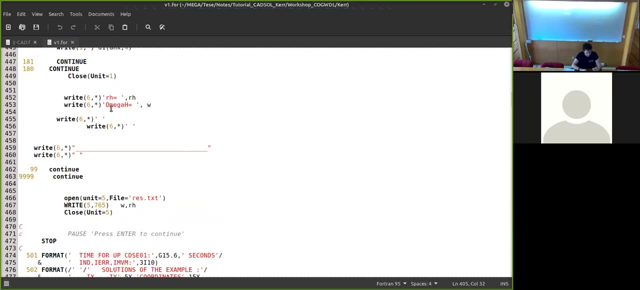 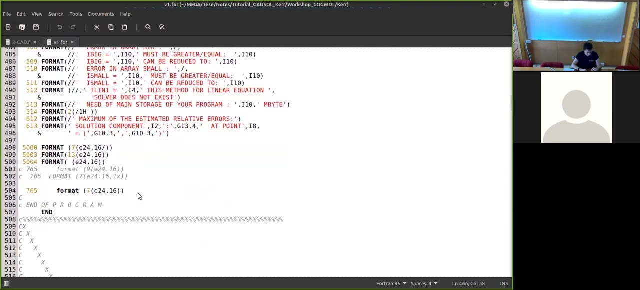 So the grid associated to the X direction and the Y direction, And here we'll print again the functions, but in a different way, And finally we'll bring to the parameters the input parameters of the problem in this res file. But yeah, 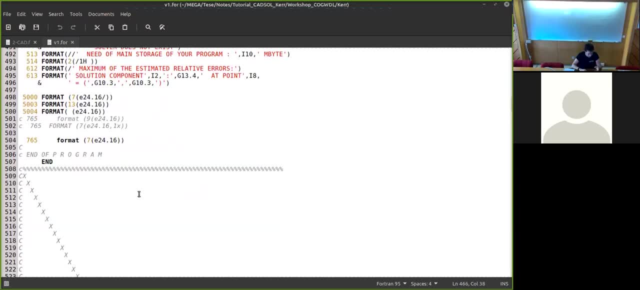 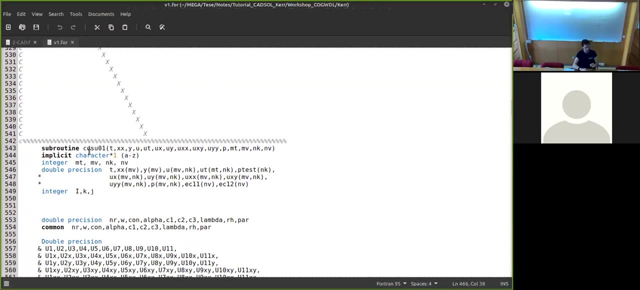 basically, this is the solver, But where do we put the equation of motion and the boundary conditions? This is put within some subroutines that are within the subroutine that we call. In this case, they are four subroutines. The first one, 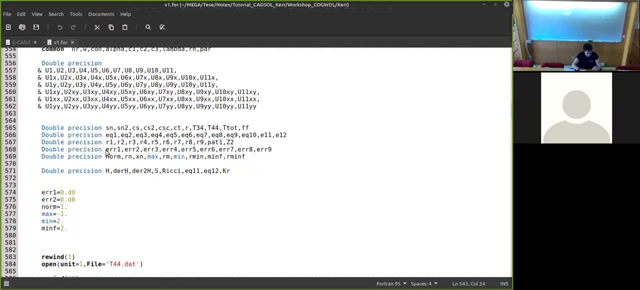 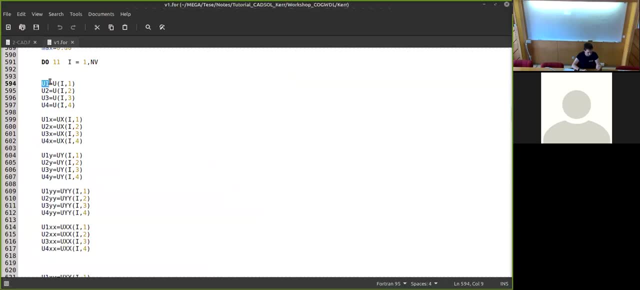 this one is where we put the equations of motion. So here first here are the definitions for the function. So F1 is F? U1,, sorry, is F1.. So in the Fortran file this is represent. 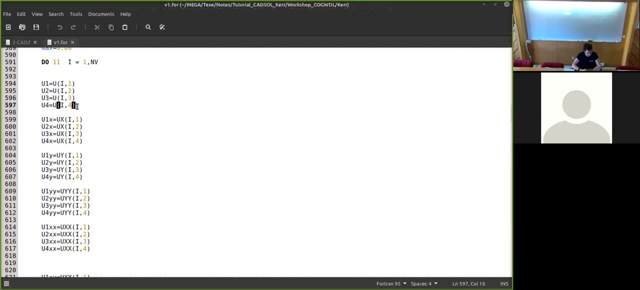 represents the first function, So it is the same for the other four. Here we have the derivatives: The first derivative in order in X in order to Y, the second in order to X and the second in order to sorry. 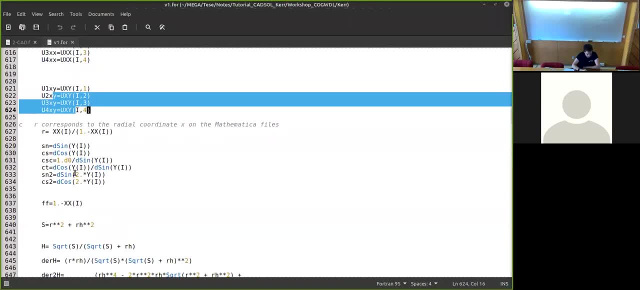 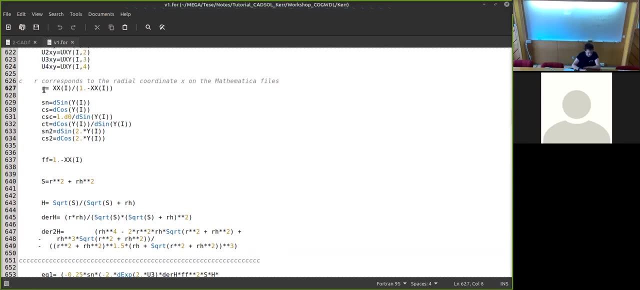 to Y in order to X and the mix. So here first we use the same terminology that we did on the Mathematica file. Unfortunately, we cannot use X here as we did in the Mathematica file, because X is used for another thing. 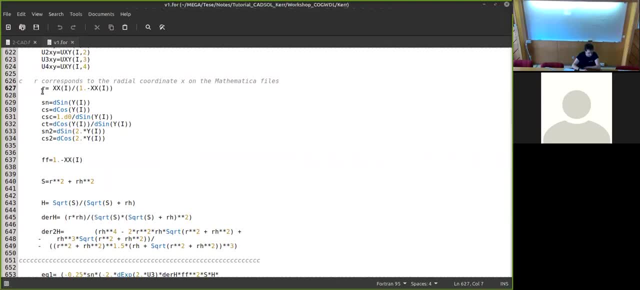 on the on this Fortran file. So we call it R. So if you want to compute, to copy the file, the equations to here, mind that that you have to change the X. You have to change the X to R. 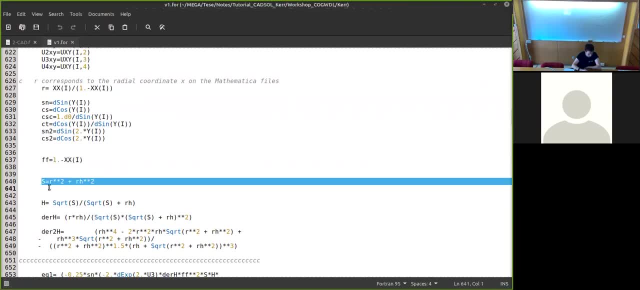 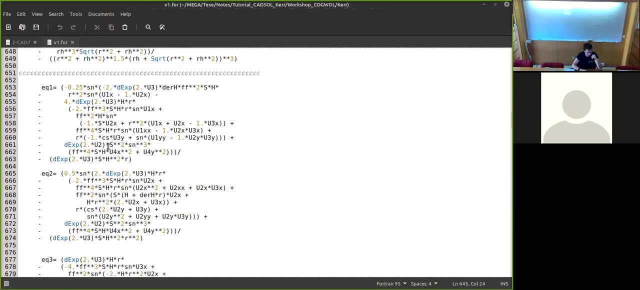 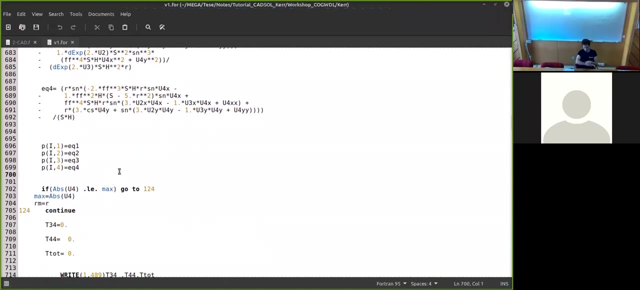 Then here we have the F function, the S function and the H with its derivatives. So you can now print or copy and paste all the equations: the equation of motion, the first, one, second and the others, The way that the solver knows that. 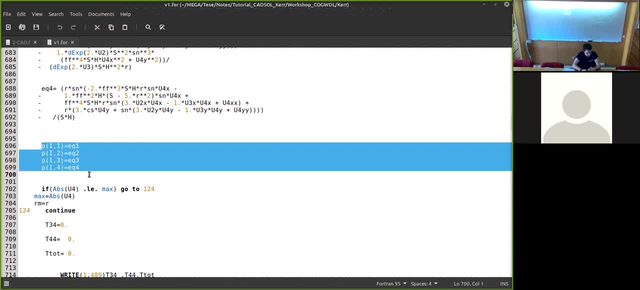 which are the equations that he has to solve, is by doing this small lines of code. So over here you're saying that, or you're saying to the solver that you want to compute the, basically the Newton residual for equation one. equation two: 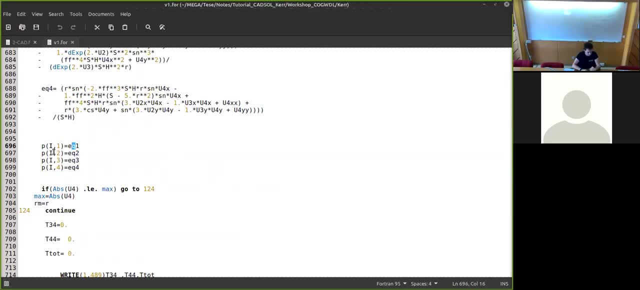 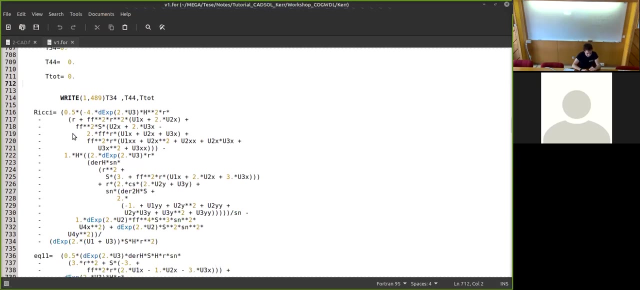 equation three. equation four: So if you want that to be as small as zero- the solver will try to solve that and try to obtain this as close as to zero- Then in this case the energy momentum tensor is zero, So it's not very important. 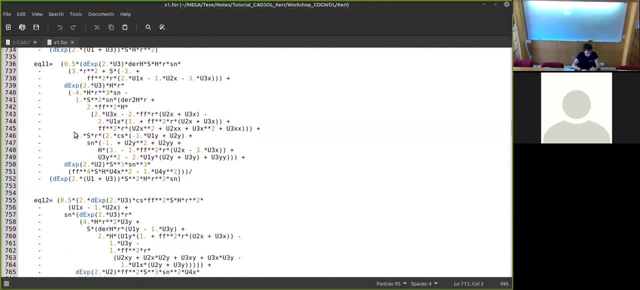 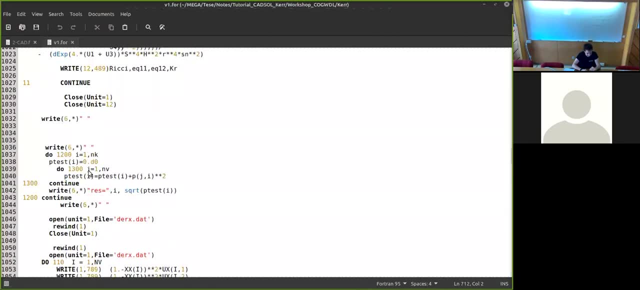 And here we also put the energy scalar, the two constant equations and the Kretschmann scalar. As you can see, the Kretschmann scalar is quite long And at the end, for these four equations, you only will compute them. 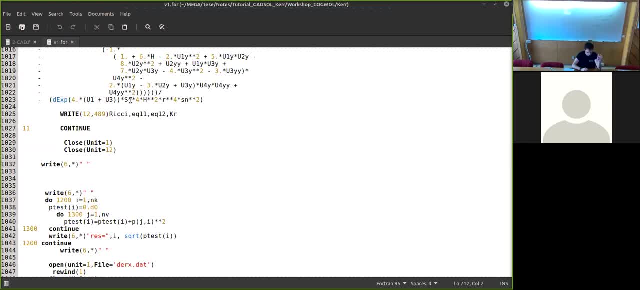 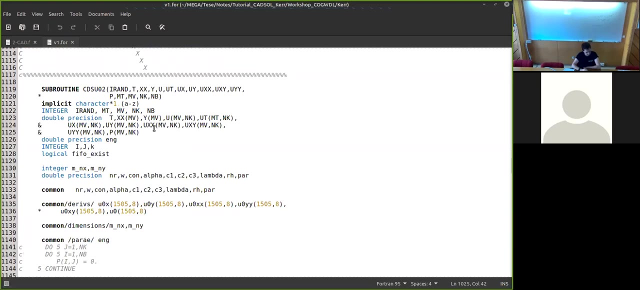 You'll not use them to solve anything. You just take the solution that he computes, substitute everything on these equations and then do a print for a FAD. So the second subroutine is associated to the boundary conditions, And here is where you'll put. 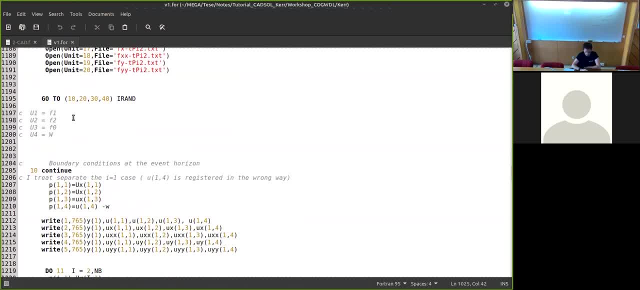 all the boundary conditions. The way that you do this is by using the go-to function of Fortran. Unfortunately, Fortran likes very. people normally like to go to use this go-to function, but it's quite annoying to understand what is happening exactly. 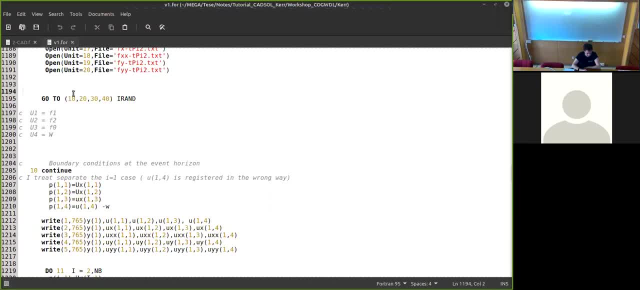 But here we have four labels: 10,, 20,, 13 and 40.. And each label corresponds to a boundary conditions, the boundary condition or boundary. The 10 label corresponds to the boundary at the event horizon. The 20 corresponds to the boundary. 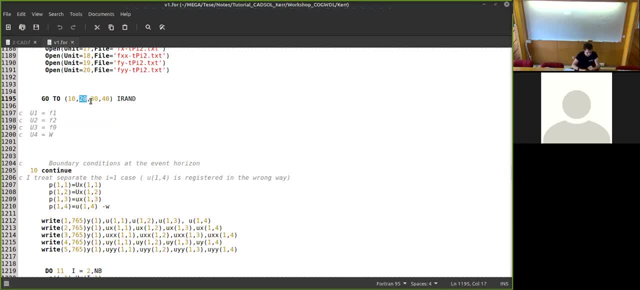 at infinity, special infinity. The third, or the 13, corresponds to the boundary at the poles, And 40 corresponds to the boundary at the equatorial plane. So for each label- so for example, here it starts the label 10, you can put the boundary conditions. 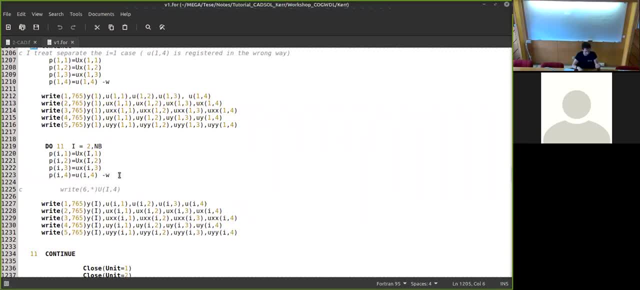 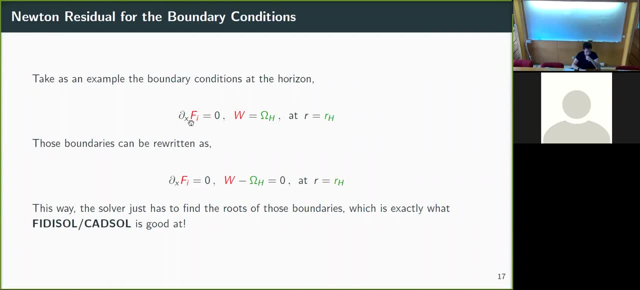 Then the way that you do this is using again the Newton residuals, which here I have an example. So at the event horizon we saw that the derivatives of the function must be zero and that W must be equal to omega H. If you rewrite this, 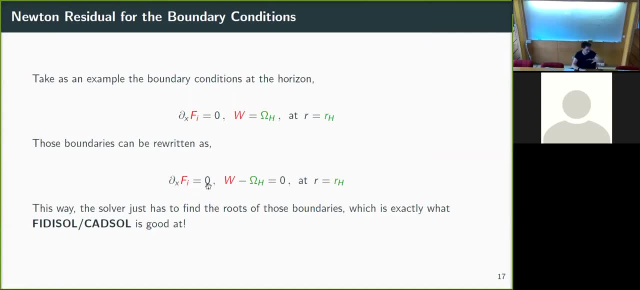 such a way that we have everything on the left equal to zero. then you just have to tell the solver that you want to find which are the function that solves this equation. Basically, try to find the zeros. So in the same way that you did. 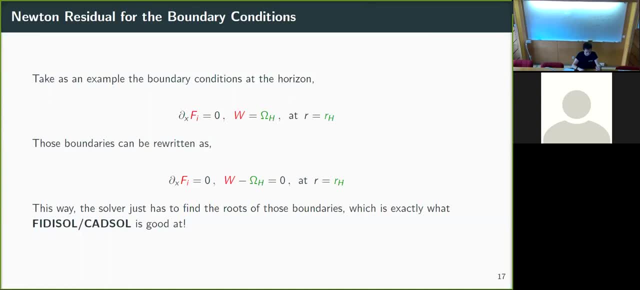 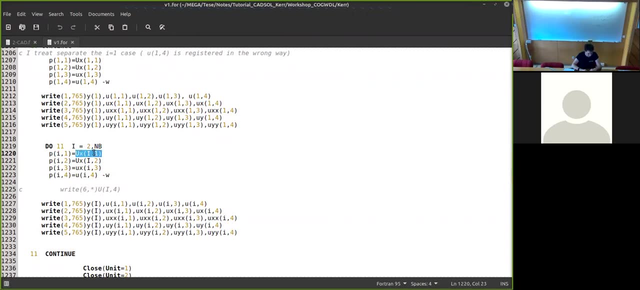 for the equations here. you can do exactly the same for the boundary conditions. That is exactly what we have here. So here we have the derivative of X of the first function That must be equal to zero. The second one, the third one. 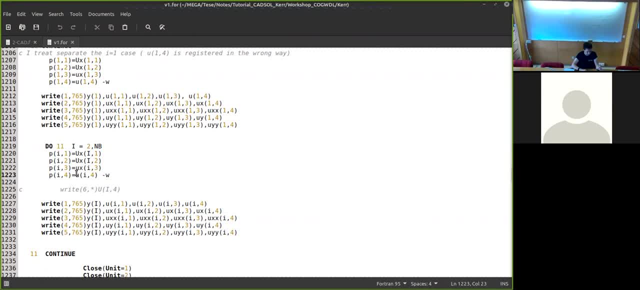 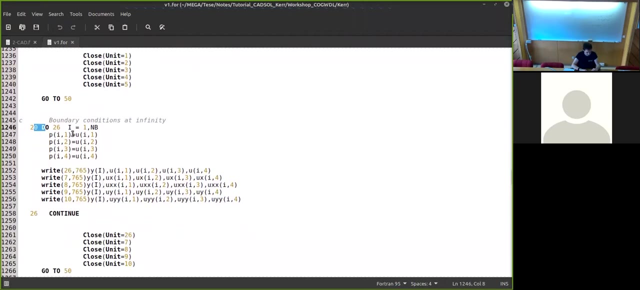 that also must be equal to zero. And here we have that the W function minus the omega H, which here we call small w, must be equal to zero. You can do this for the other boundaries. So here for the infinity boundary that all the functions must be zero. 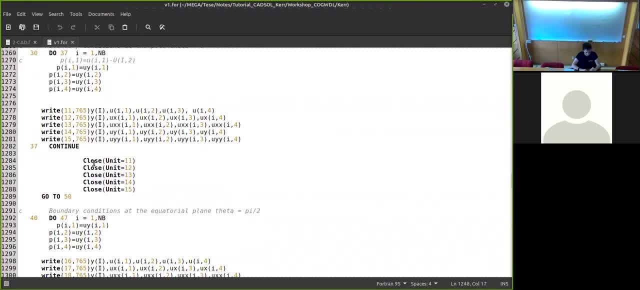 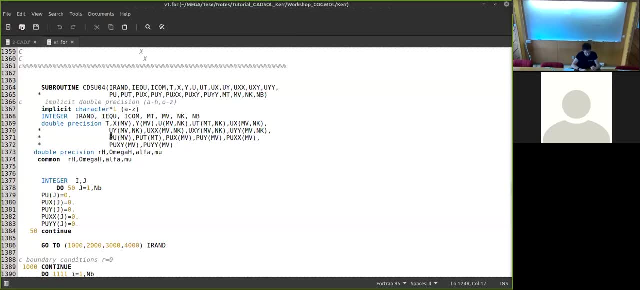 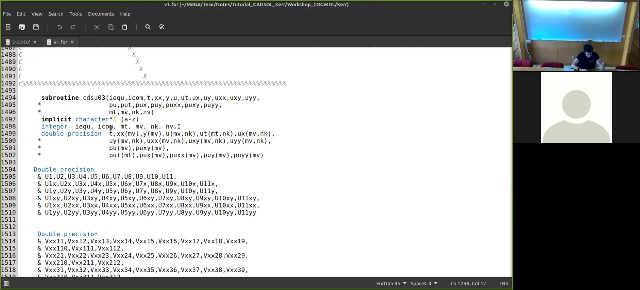 So it is, And you can do again for the poles and the equatorial plane. Now here is the fourth subroutine, but it's not very important so I will not talk about it. But then we have the third- sorry, the third- subroutine. 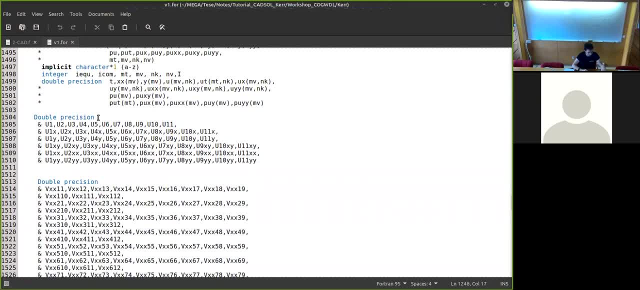 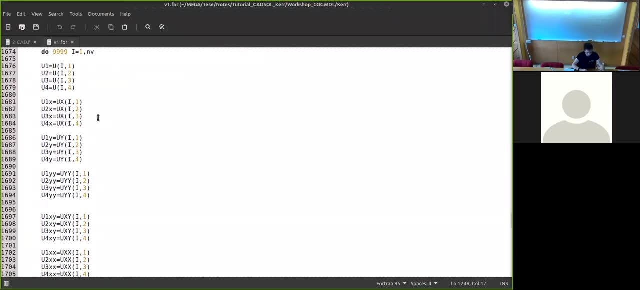 in which here is where you put the Jacobian matrices. So, as you can see, that will be quite a pain to copy everything and put everything. So here we do, the same for the functions and the same for the YAR variable, the FF. 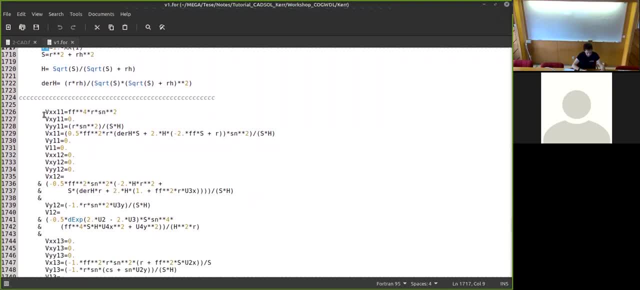 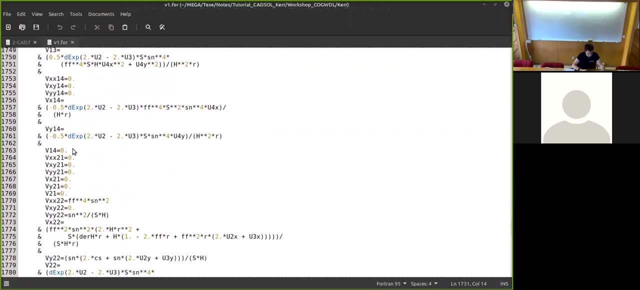 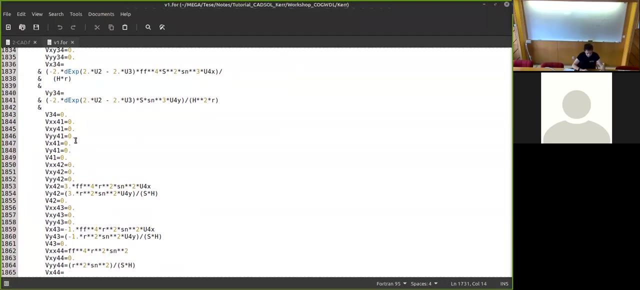 the X and the H functions, And here is where you start to put all the entries of the matrices. So, as you can see, there's a lot of them And most of them are zero, so it's a bit easier, but it's quite. 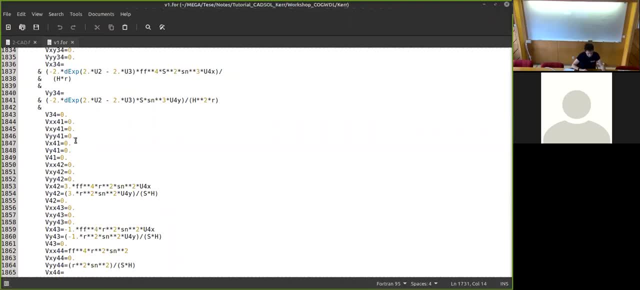 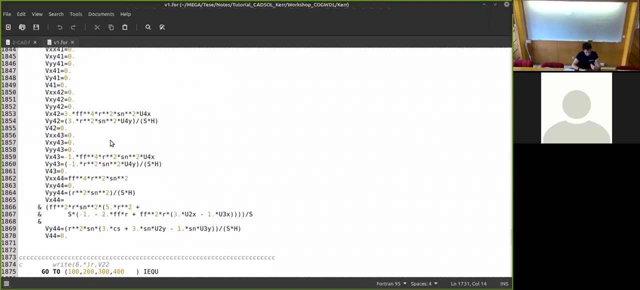 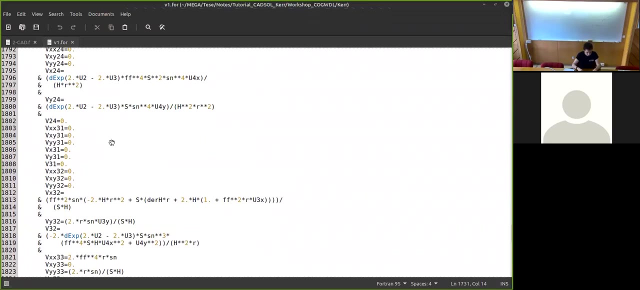 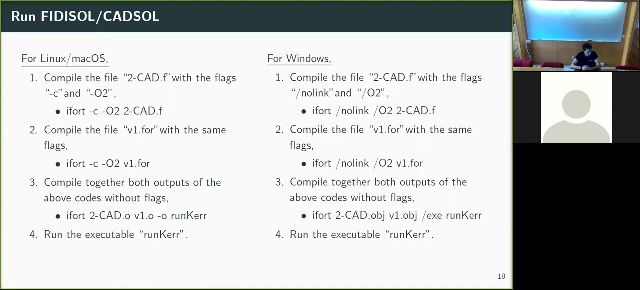 it's quite painful. Well, it takes a while to put this, put every single equation here, But when you finish this, you basically have everything done. So you just have to run the code And for that, depending on which OS you are using, 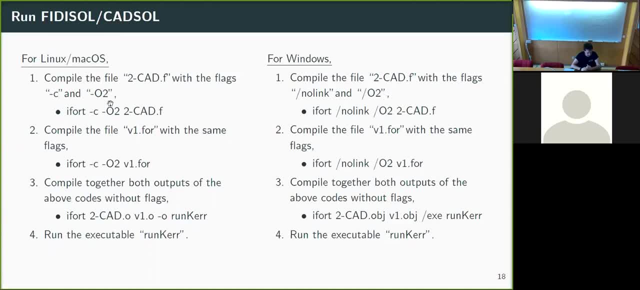 for example, for Linux and macOS it's the same. I didn't check for macOS, so if I'm wrong- sorry, I don't have a macOS to test that- But at least for Windows, and for Linux and Windows, this is correct. 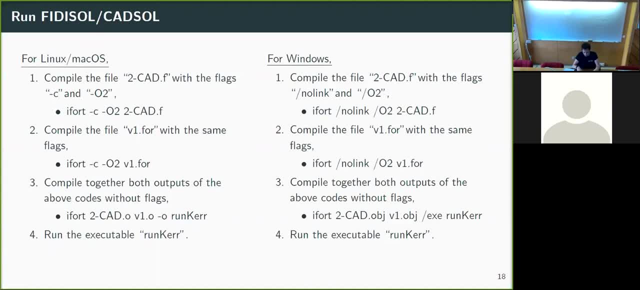 At least when I try it on my PC, which has Windows, and my desktop at home it has Windows. it worked. So to do this you just have to run these three lines of code. First, you run the brain of the operation. 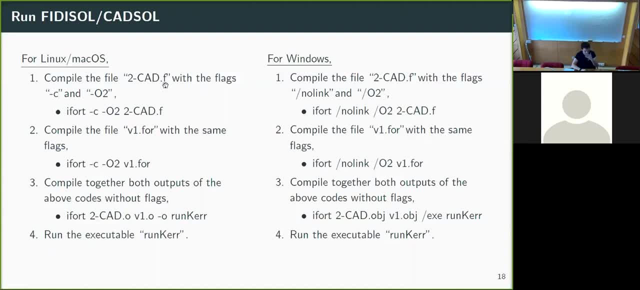 the toCADf file and use two flags. The first one, the slash C, is a flag to not link the outputs. Basically, what this means is that when you compile, you'll get an output file which, in the case of Linux and Mac, is 0.0. 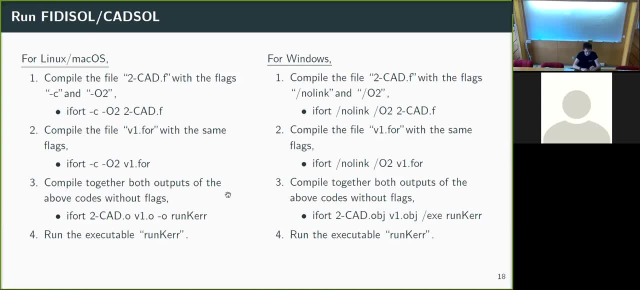 In the case of Windows it's object. So basically it's an object, It's not an executionable file. With this you can then use in this line that output to run everything. This O2 flag is just an optimization flag. 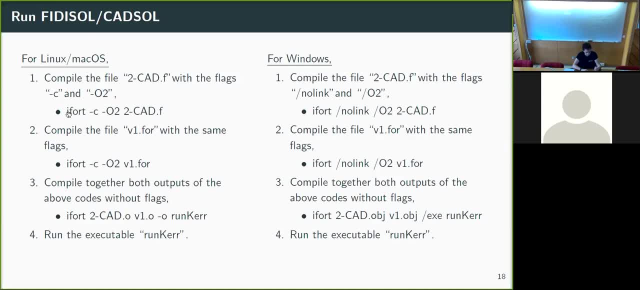 By default. the iFortum already does this, So you could omit this. It's not very important. Then you do the same for the V1 file, which is the file that we altered, and we put everything there. We do the same. 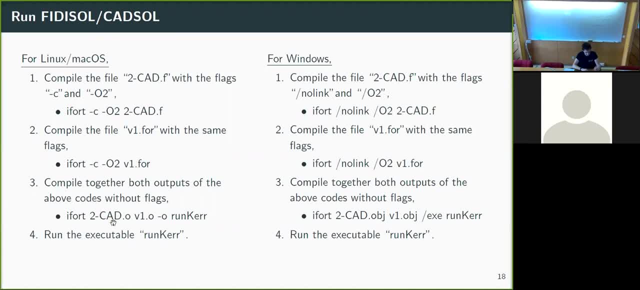 And with those two outputs, the os or object files- we run those two together And then we link them together basically and we output this as executionable. So then you just have to basically run that file. So I'll show you how to do this. 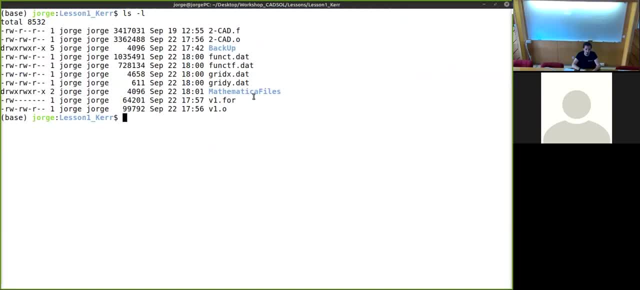 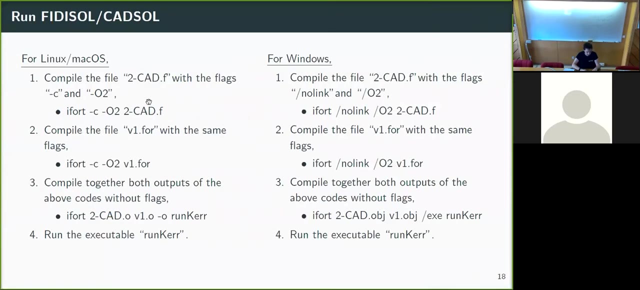 So here I have the, the two files, the two Fortum files, this one and this one. I already have the outputs from the two initial codes, these two. This one will give you some warnings, some remarks, but it's not very. 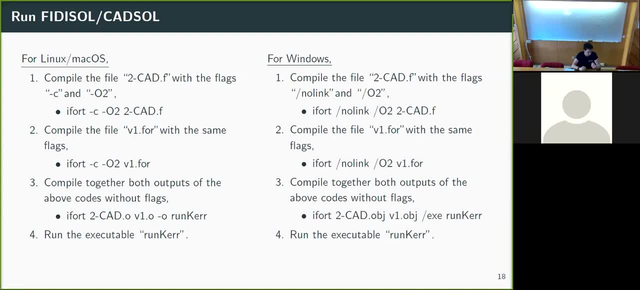 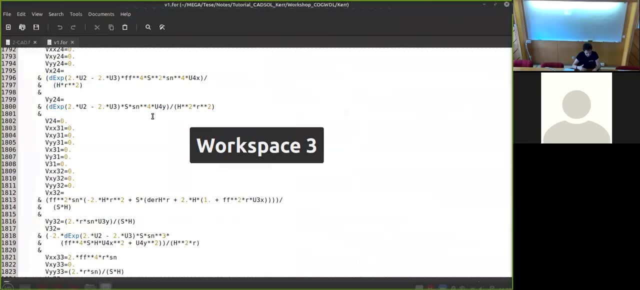 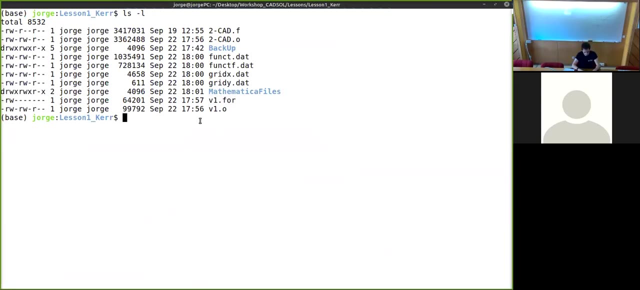 you don't have to be worried about that, Unless if you get an error. that's a different case, But it takes quite a while, So I will not run here Then for the V1 file. it should be quite fast Then with that. 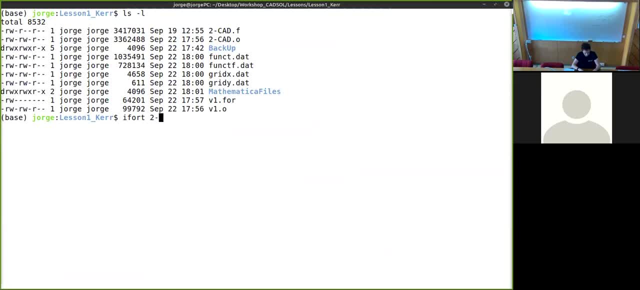 you can do iFortum with the outputs And you will have an output which here I call it run curve. If you did this, sorry for in the case of Windows, I forgot that. Oh, sorry For case of the Linux. 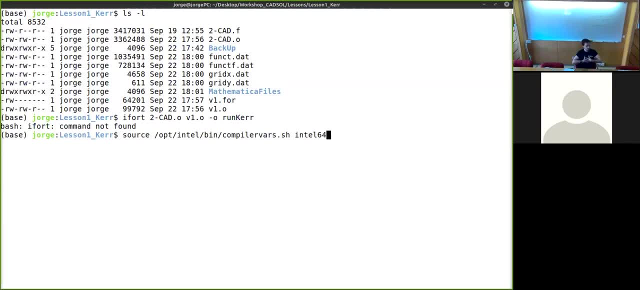 when we install this compiler we have to source some variables within the Fortum compiler. So you have to run this code, everything you open a terminal to be able to use the Fortum compiler. So you can now run and hit run. 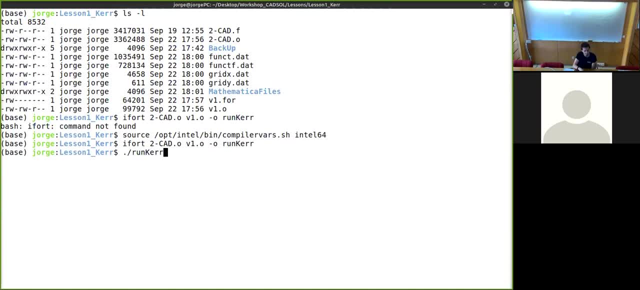 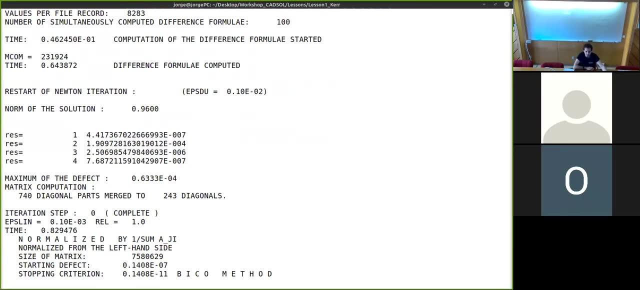 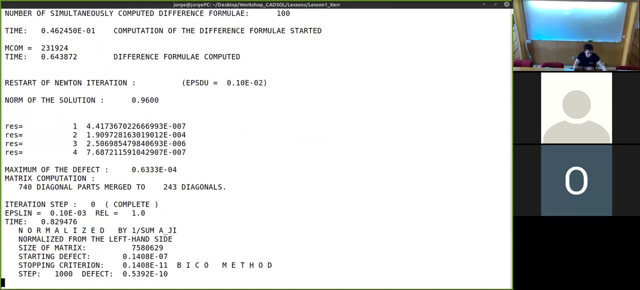 So you just have to now run this executable Doing this, sorry, sorry. yes, You could just add it to a bash RC, right? Yeah, it's true, It's true, Yeah, it works, But yeah, I didn't do it myself. 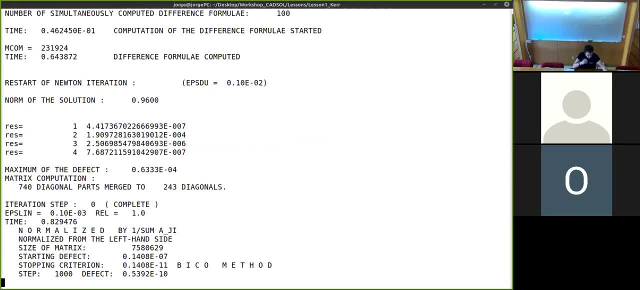 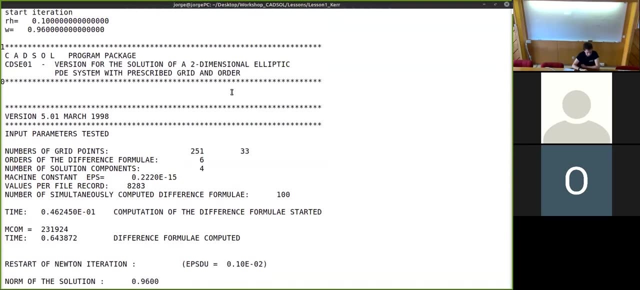 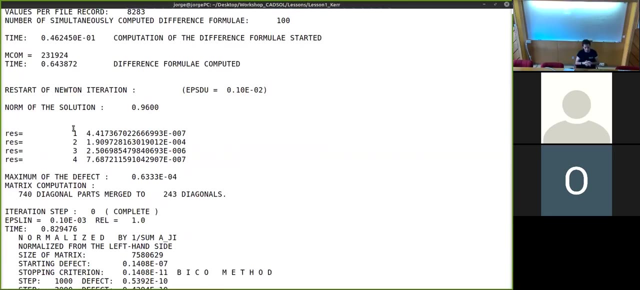 But yeah, you can do that In principle it should work. Okay, good, Thank you. So this is the output of the cat solve. So there's some parameters in the beginning. So there's a lot of information here, But the main points: 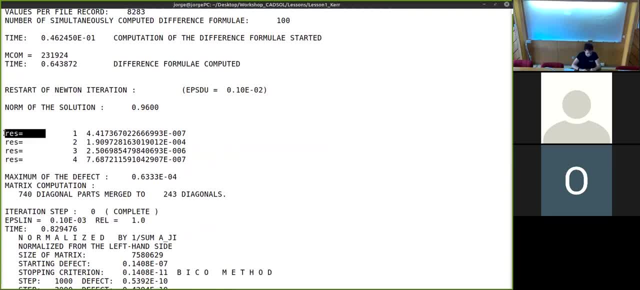 that I want you to focus on is first on this, which is the Newton residuals. As they are the Newton residuals, they should be close to zero And, as you can see, this is already very close to zero. This also happens here because we are using 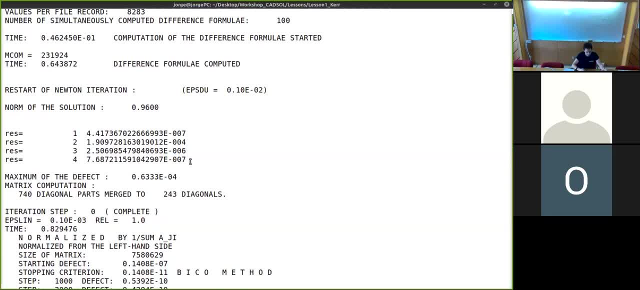 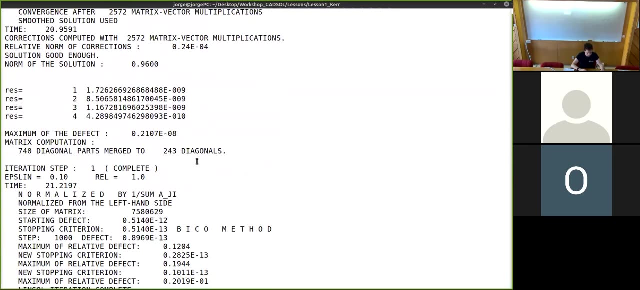 the exact solution as initial guess. So usually you will not have minus seven or 10 to the power of minus seven. on the first iteration And in principle after the third iteration you have quite good results. Then we can also look at: 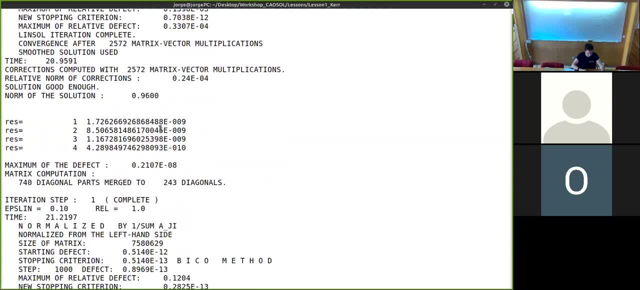 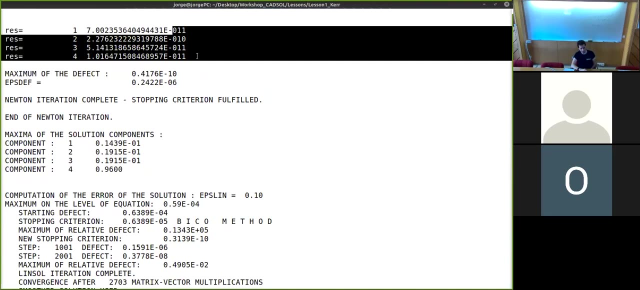 for example, now that the solver ran a bit more, as you can see, the residuals are a bit better. So 10 to the minus nine and 10 to the minus 10.. And here you get to the minus 11.. 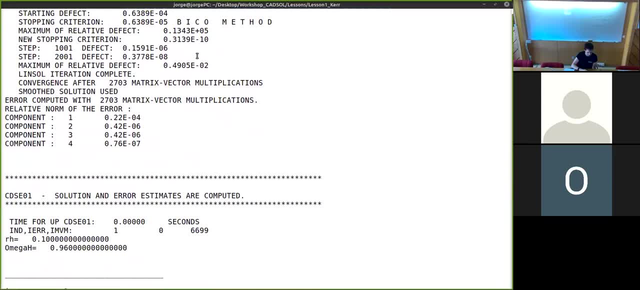 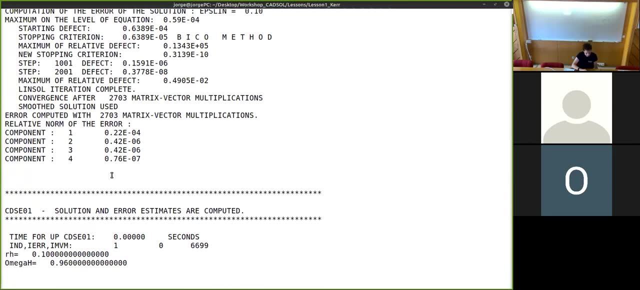 So the second one here. it ended the first iteration, So you will also do the second in the third iteration. But let's look at this. The second thing that I want to look is basically this: It says that the solver computed the solution. 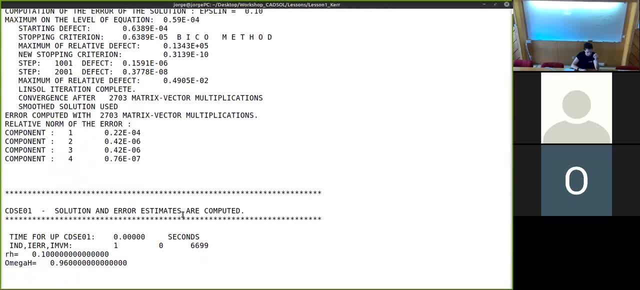 and also provided the error. So if you run it and you get this expression, this phrase, then in principle everything is good. The third and last part that I want to show you, I want you to look at, is the relative norm of the errors. 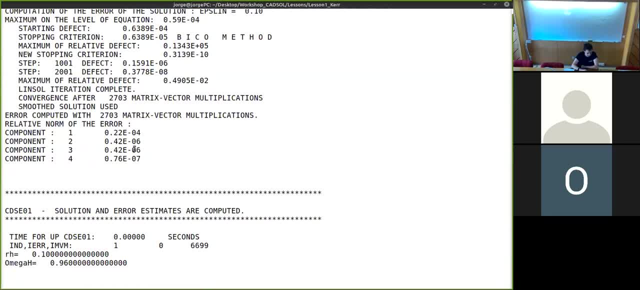 So basically this: This is basically the errors estimation for each function. So F1, F2, F3, and W. Sorry, F1, F2, F0, and W. So since this is an error, you expect to be. 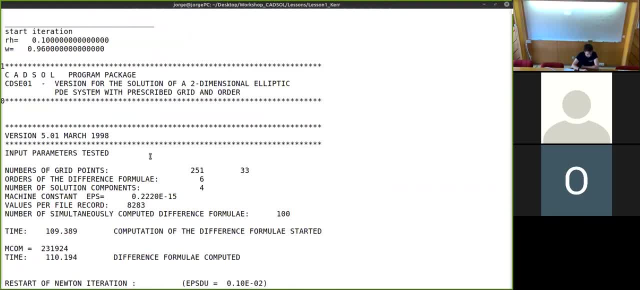 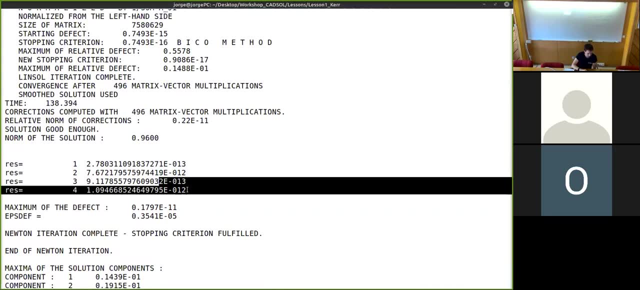 close to zero. So now I can show you the last iteration. So it's still finishing. So on the third iteration you can see that the residuals are a bit better, but it starts to get to a point that it cannot get any better than that. 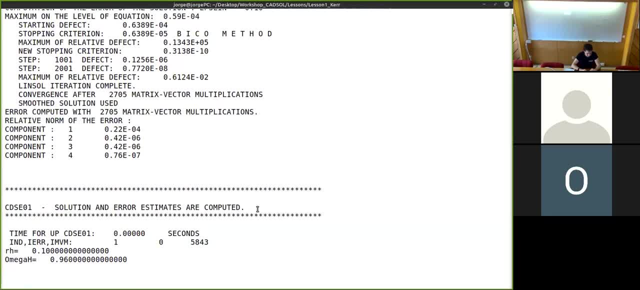 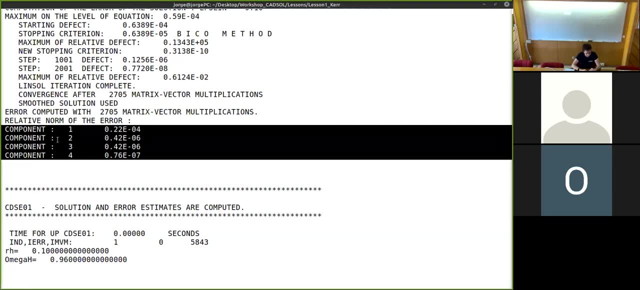 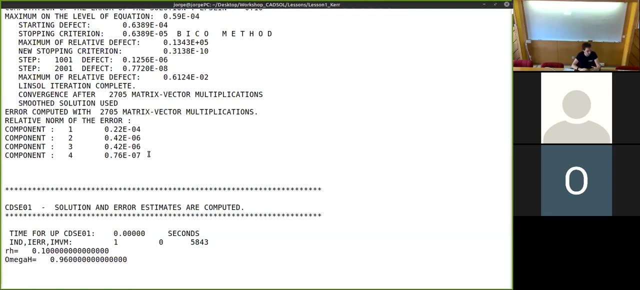 And it finished for the third iteration And, as you can see, everything went well And the result of the relative norm of the errors, as you can see, didn't change much. So this is basically the best you can get. So that's basically it. 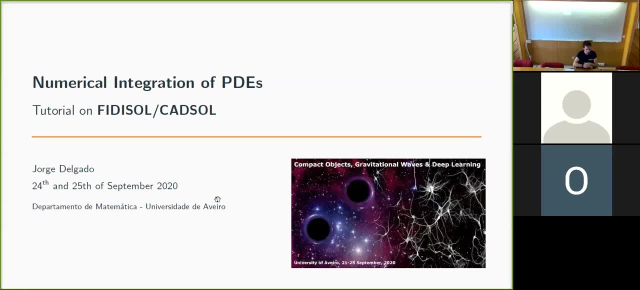 That's what I have to show you in this first lecture. If you have any questions, please do so. Tomorrow's lesson, I will give you some solution of a Boson star, of a rotating scalar Boson star, And we'll start to see. 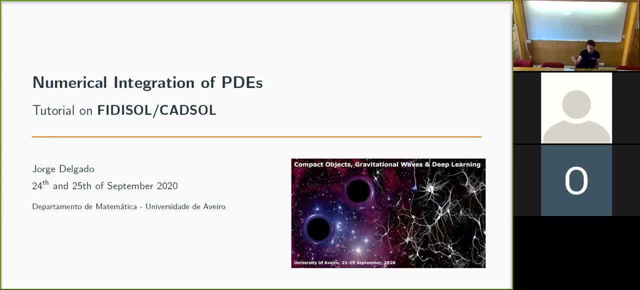 how to obtain some physical quantities such as mass and momentum and other quantities. So, thank you, Thanks, Jorge, Thank you very much. Thank you very much, Jorge. I think we will have quite a. It's almost a factory, Basically. 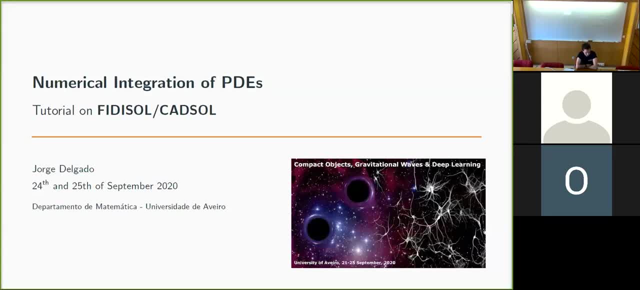 It's very social. It's really nice. Yeah, So questions- Online questions. I don't see questions in the room. It means that we are very clear. You can continue Right at the beginning. what was the criteria for the choice? 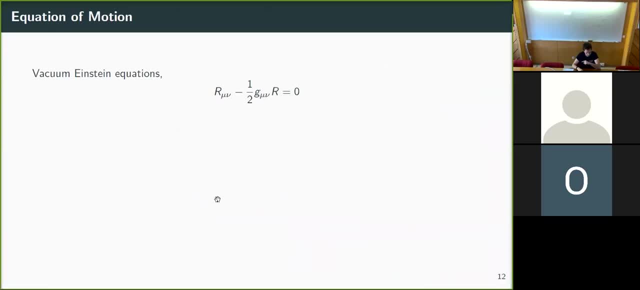 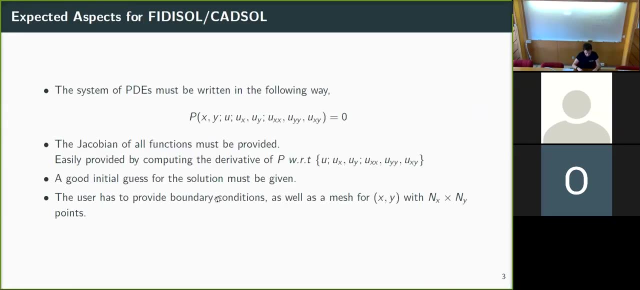 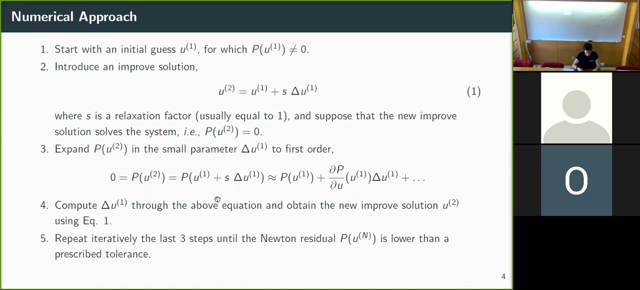 of the relaxation parameter On the file or the On the slides, On the slides. Okay, So we are introducing the method, The method. So you were talking about the. So Yes, Yes, Yes, Yes, Yes. 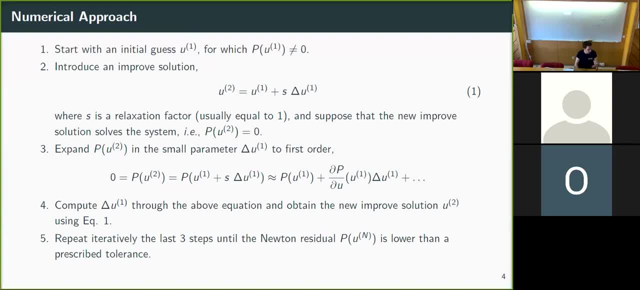 It's a relaxation factor. It's basically always equal to one. It's not very, very important. But what this does is basically like the learning rates in the In deep learning. Basically, you are doing: You take one solution and if you want to jump,